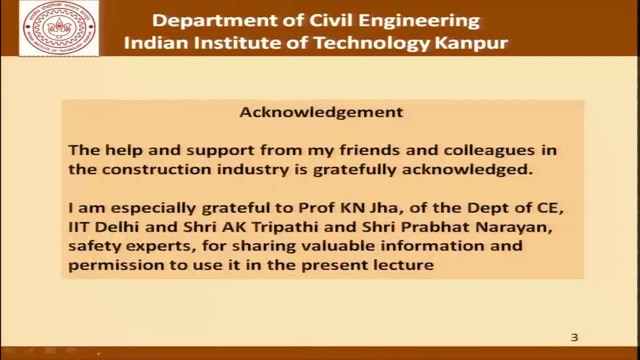 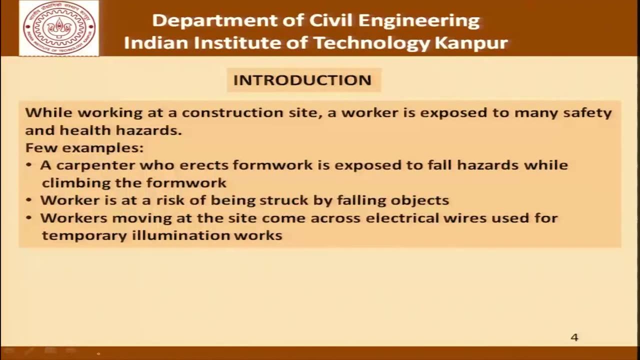 in different places, And I would also like to thank the members of the country for sharing the valuable information and having given me permission to use some of the material and some of the information in this present lecture and also in this module. Now to get started. while working at a construction site, a worker is exposed to many safety and 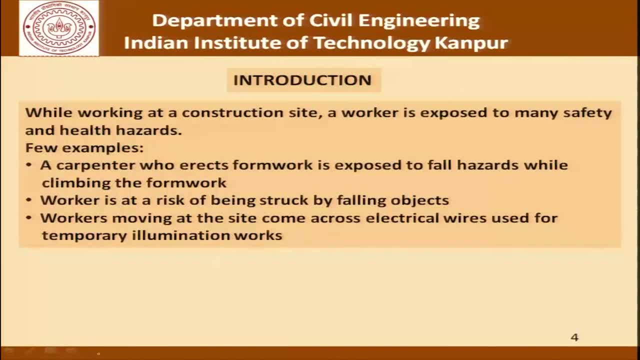 health hazards. Some of these examples could be: a carpenter who erects farm work is exposed to fall hazards. while climbing the farm work, He may be at risk of being struck by falling objects. He may just be walking on the ground and there may be work going on at a height and a nut or a bolt or a screwdriver or whatever. 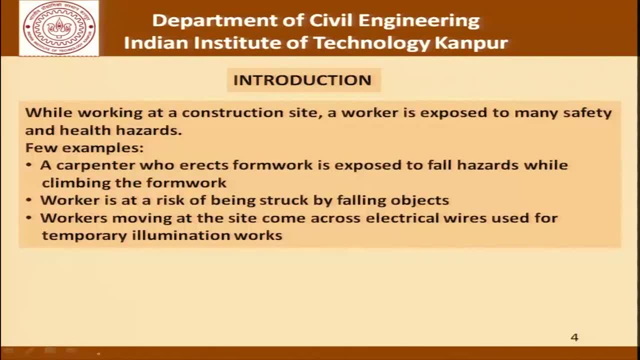 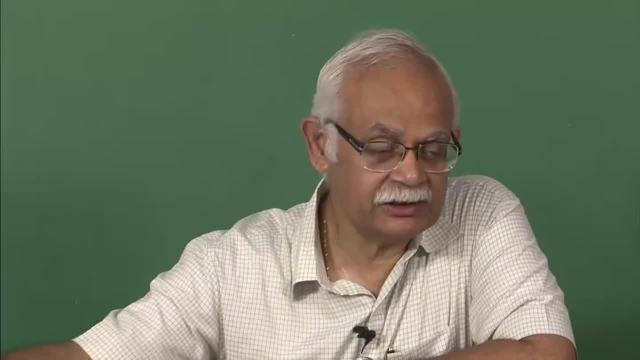 it is may simply fall and hit him on the head. It may not be a worker. in fact it could just be a passerby. This happens very often when we are trying to do construction work in built environment in urban areas. Workers moving at the site come across electrical wires used. 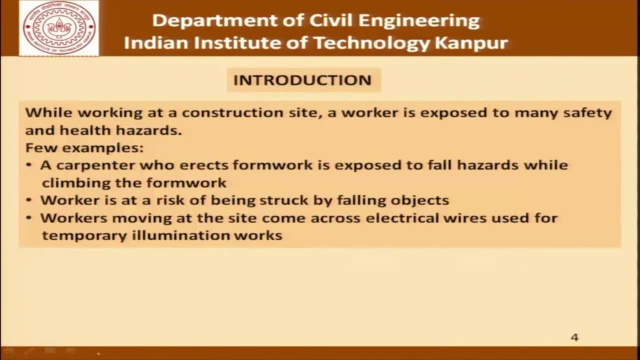 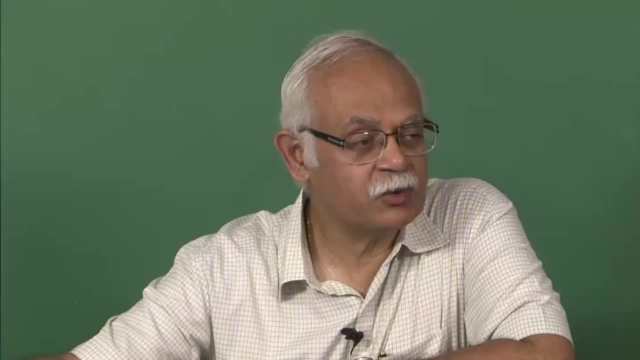 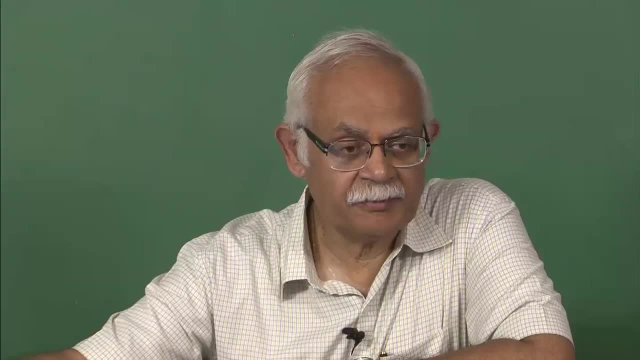 for temporary illumination works. They can trip on those wires, The wires can cause a short circuit and cause a fire, and so on. If you are working in marine environment or near the water, there is always the possibility that the worker may fall in water and there is a drowning issue involved If there are 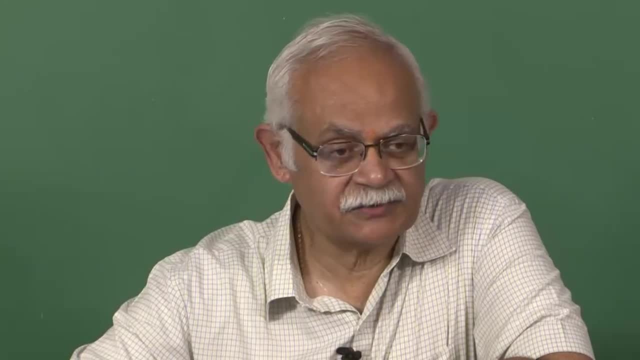 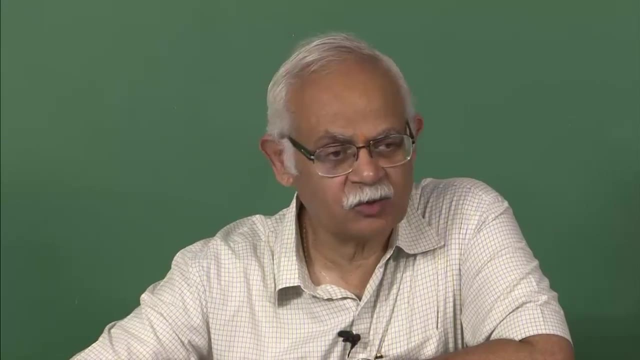 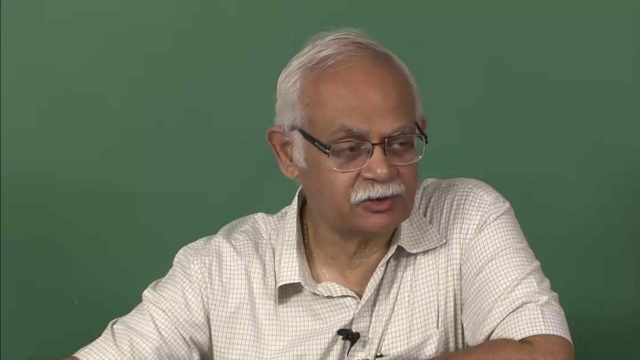 operations like welding being carried out, there is an entirely different set of hazards that are faced by construction workers. We do not want to have accidents at site and it is an important responsibility as far as the construction manager is concerned to ensure that the construction site is accident free. 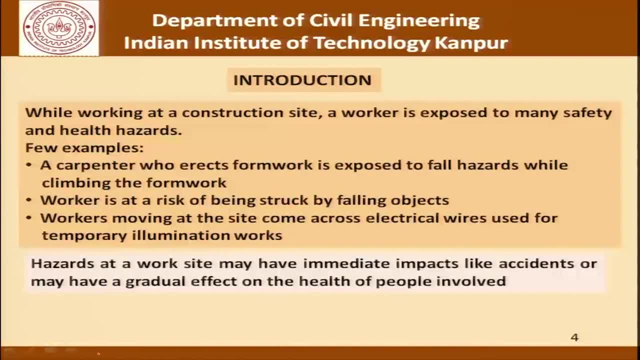 Hazards at work site may have immediate impacts, like accidents, or may have a gradual effect on the health of the people involved, and that is why we often deal with accidents and health hazards together, And the environment is often called HSE, which is health, safety and environmental. 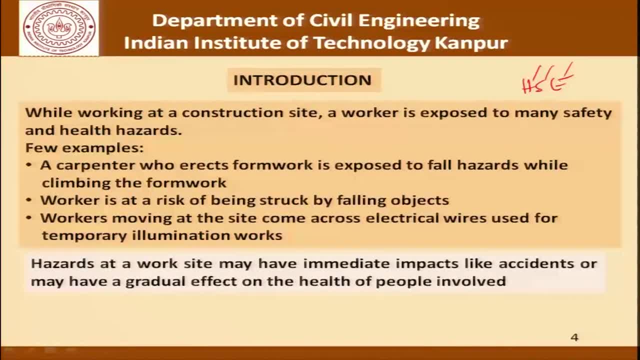 safety. So these three things are very closely linked to each other and are often held together as far as the corporate policies are concerned. In fact, even regulatory authorities like the OSHA is the Occupational Safety and Health Administration. This regulatory body, which is a US regulatory body, deals with occupational safety and health As far as construction. 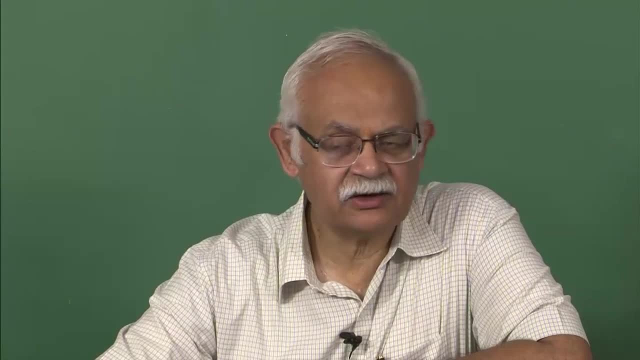 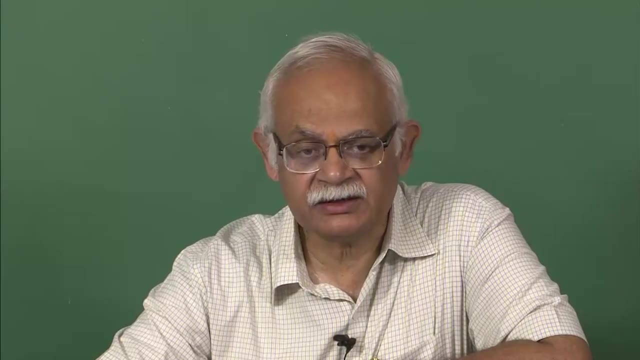 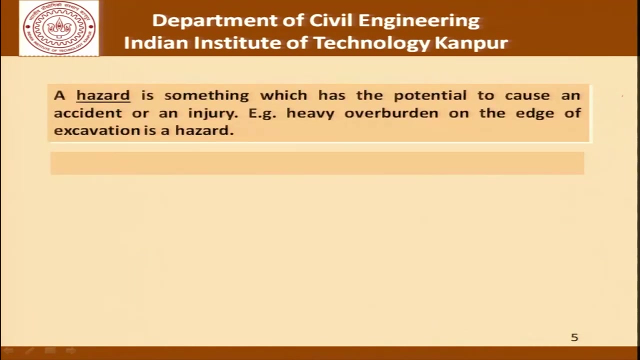 workers are concerned. construction is their occupation And all that environment they basically involves concerns about their health and their safety. so before we move further, we should try to have more precise understanding of some of the words that we will use. a hazard is something which has the potential to. 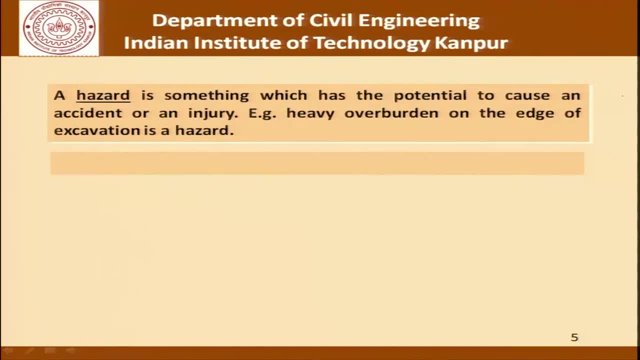 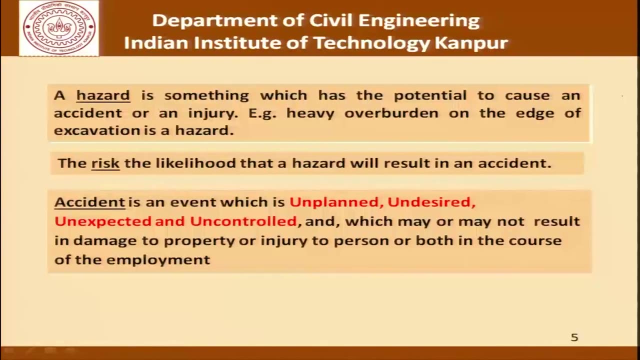 cause an accident or an injury. for example, heavy overburden on the edge of an excavation is an hazard. the risk is the likelihood that a hazard will result in an accident, and the accident itself is an event which is unplanned, undesired, unexpected and uncontrolled, and which may or may not result in damage to. 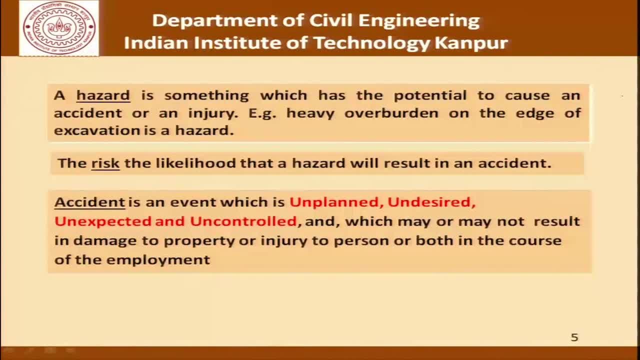 property or injury to person, or it may result in both in the course of employment. so these four words- unplanned, undesired, unexpected and uncontrolled- these are very important to understand. in the context of an accident, all effort as far as safety is concerned is directed towards. 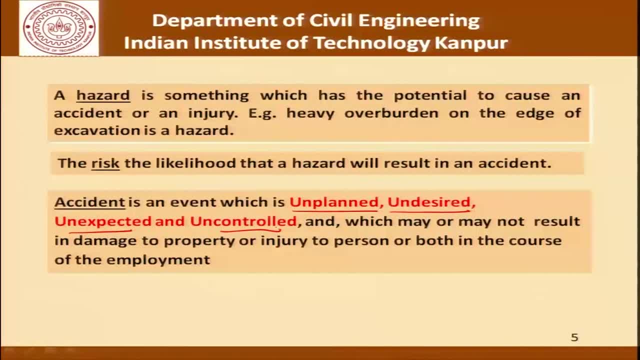 you, reducing the chances or the probability of an accident occurring at sight because it is uncontrolled. at the end of it, sometimes we really do not know what would be the result of an accident. it could be something which we just not foreseen. now, before we go further, I would like to share with you. 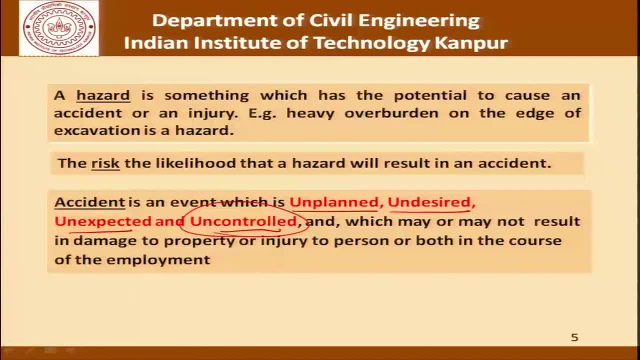 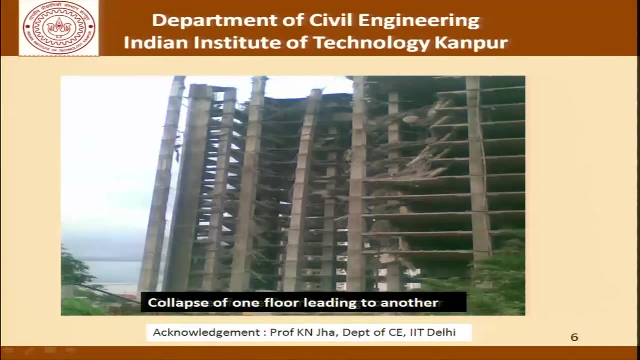 some of the photographs of construction related accidents and, obviously, a civil engineers. we cannot be proud of them. these are something which is a very, very difficult situation for us to reconcile with, and we must leave no stone unturned in ensuring that these kind of things do not happen at sites where we are in charge. this picture here. 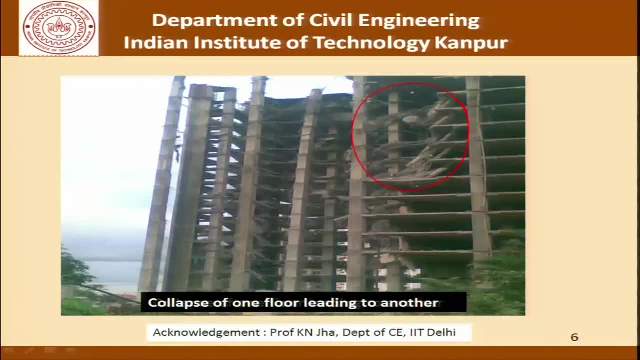 is the collapse of floors in a multi-story building. now, how that happened, why that happened, is a different matter. the fact that some of these floors have simply collapsed while the building is under construction is a matter of great concern. it could have happened because of faulty materials. it could have happened because of faulty designs. it could have. 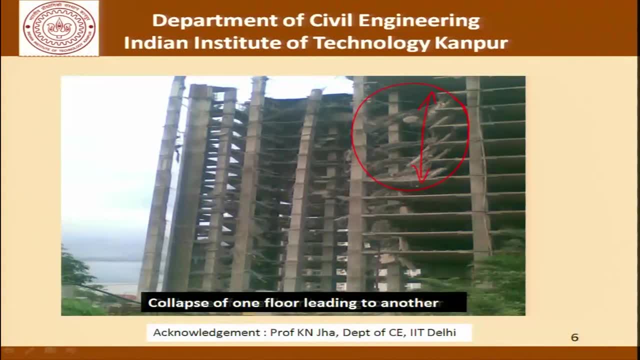 happened because of faulty or bad workmanship in terms of erecting formwork, removal of formwork and so on, and that is exactly what is the issue. construction safety involves handling these things, learning lessons from them and ensuring that the accident is not repeated. this is another accident where 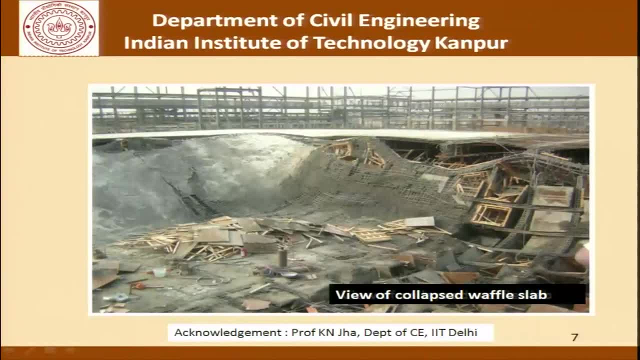 we can see the collapse of a faithful slab, so we can see that once an accident happens, there's so much of reconstruction that has to be done. there is so much of loss that has happened that it's very, very difficult to recover from that. the cost of an accident is simply very high. those are things which 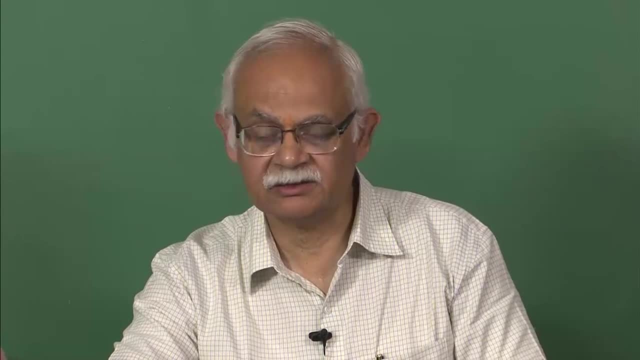 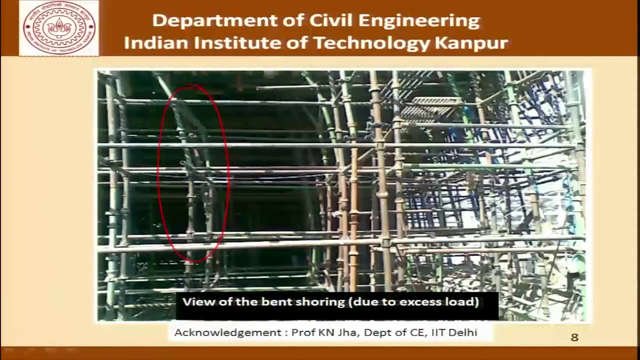 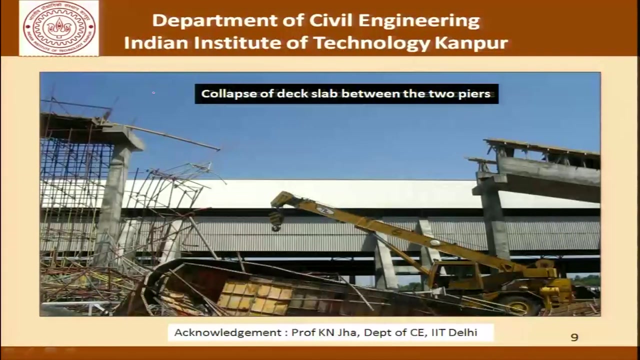 we need to talk about and at least be aware of as construction professionals. this picture here shows bent shoring. now this bent shoring could be on account of excessive loading. this is a view of a collapse to deck slab between two piers. this picture here you can see the sky, because 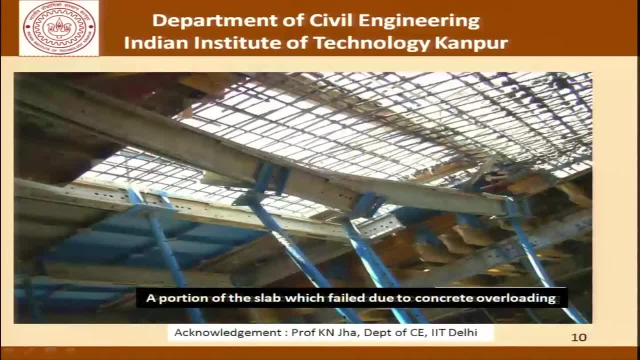 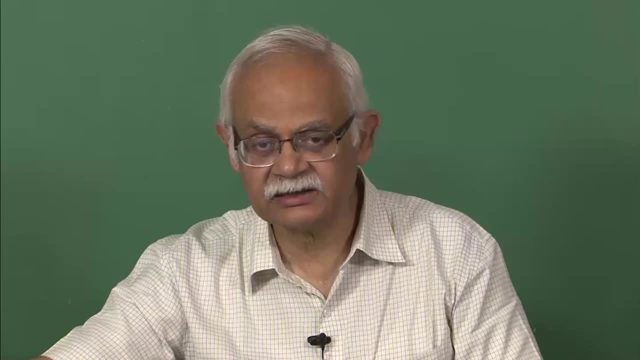 the slab between the two piers has simply collapsed, a portion of the slab which failed due to concrete oak loading. now there's no question of overloading as far as the structure is concerned. the structure is not even in service. if the cause is overloading, then it is loads while construction is going. 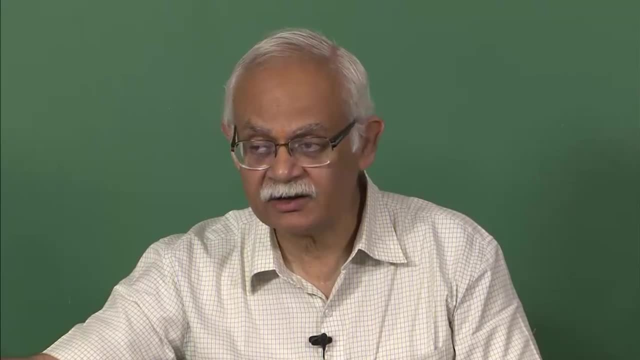 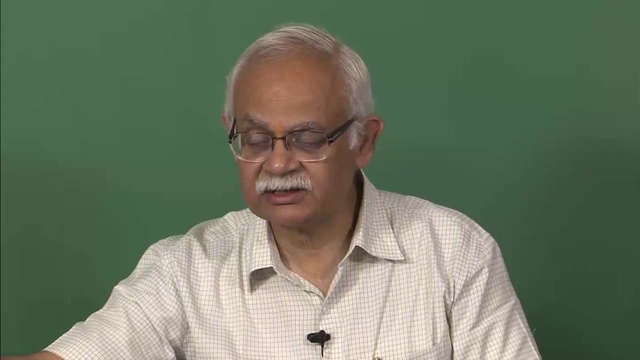 on at that time we must remember that the concrete may not have achieved full strength. So we have to be very careful and plan for what are the loads that are likely to come on the structure while it is being built and make sure that concrete at a given 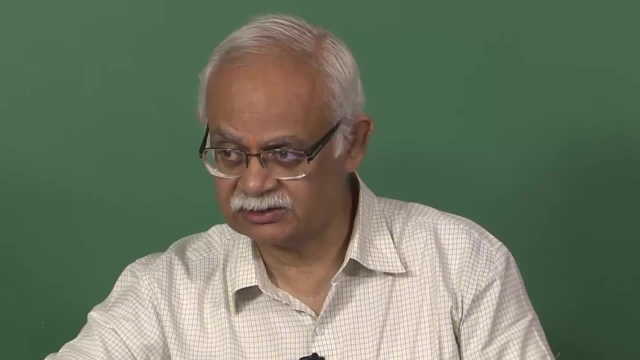 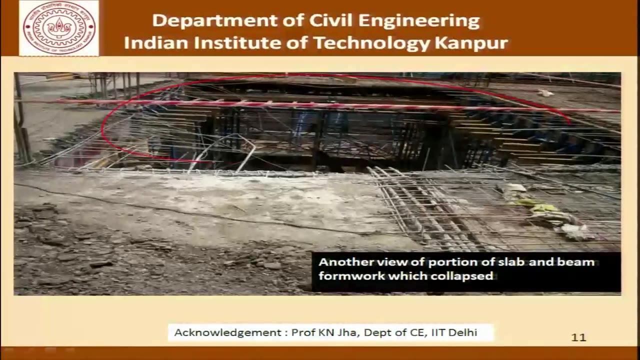 point in time, has sufficient strength to withstand those construction loads. Here is another view of the portion of the beam and slab formwork that has collapsed. So here is the entire slab which has just caved in. Here is the picture of the failure. 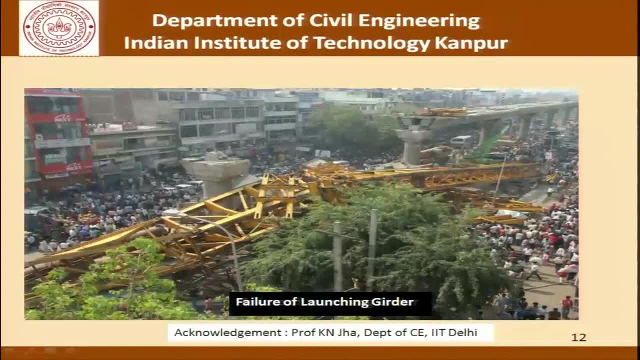 of a launching girder. You can see that working in built up areas has its own challenges. it has its own implications in terms of consequences of failure, the effect on passersby and so on. Now this is yet another picture of an accident where there is a metro bridge span. 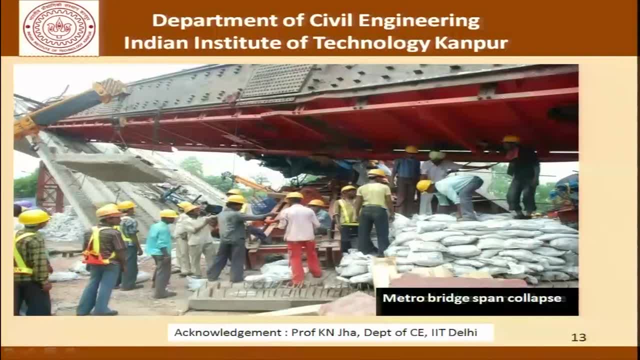 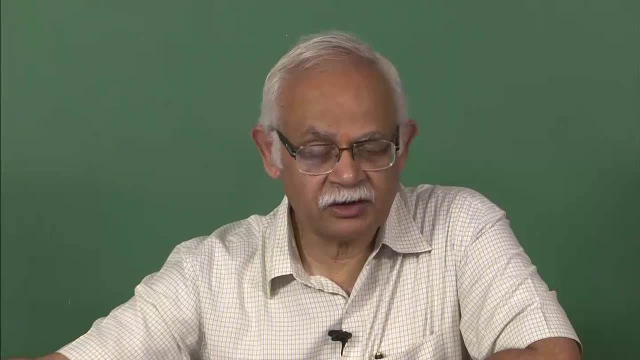 that has collapsed. The intention of going through some of these pictures was not to discuss the accidents or discuss the causes of those accidents, but just to show you that construction accidents are very, very painful to see. 00. They are very painful to investigate, but yet it is important that a construction manager 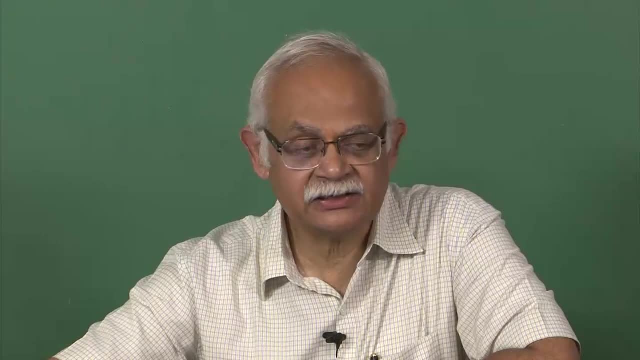 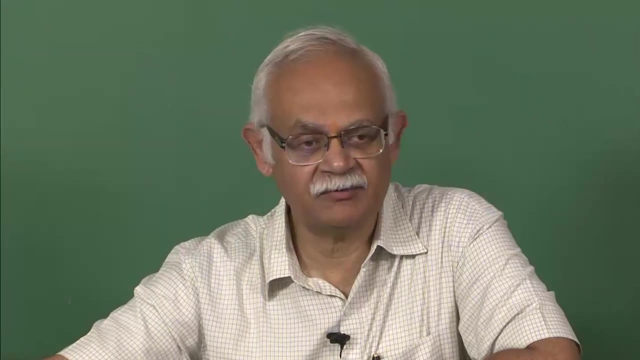 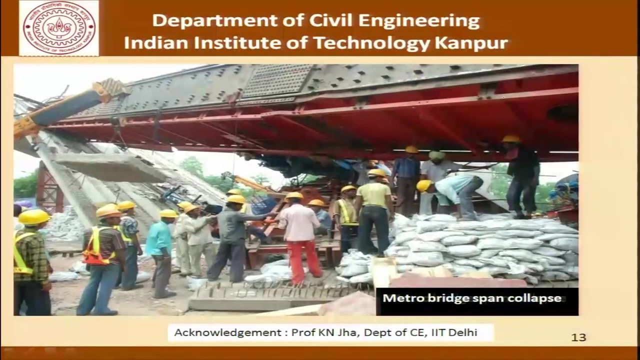 understands the issues involved in construction safety and take steps that accidents do not happen at their site, And if each manager ensures that, we will indeed have a accident-free construction industry. With this, let us try to move on to some more discussion as far as construction safety related. 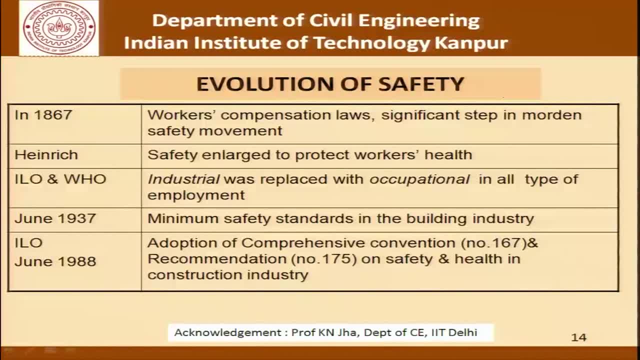 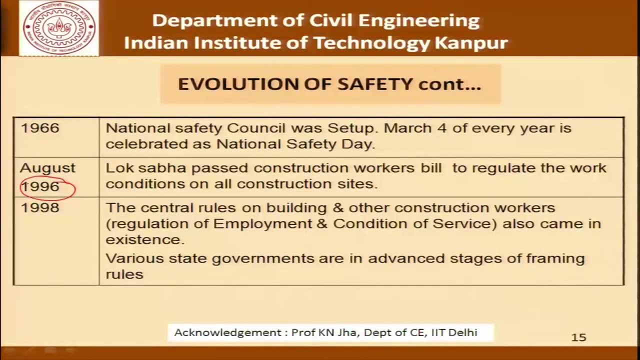 issues are concerned. This slide here shows how, over the last about 150 years, different aspects of construction safety and industrial safety have evolved as far as the world is concerned And as far as India is concerned. it was in 1996, which was a milestone, when the Lok Sabha 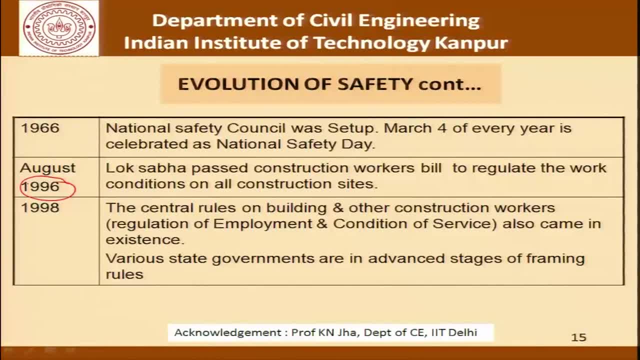 passed a construction workers bill to regulate the work conditions of all construction sites, And the central rules on building and other construction workers, called the BOCWA, came into effect, And various state governments are now in advance. These are the stages of framing the rules, and I will leave it to you to try to understand. 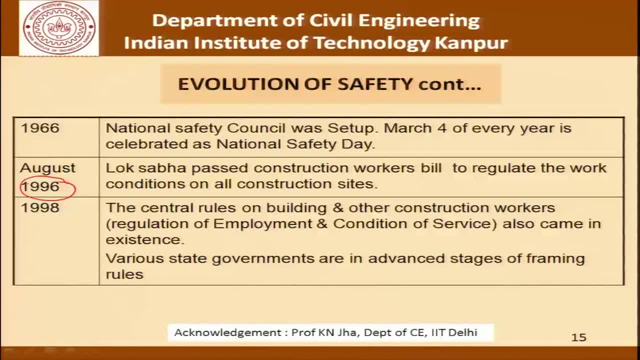 or try to do a little bit of search and find out what these rules are. We will talk about it a little when we are talking about legal issues related to construction and also, what are the provisions? which are the states that have implemented them in India? 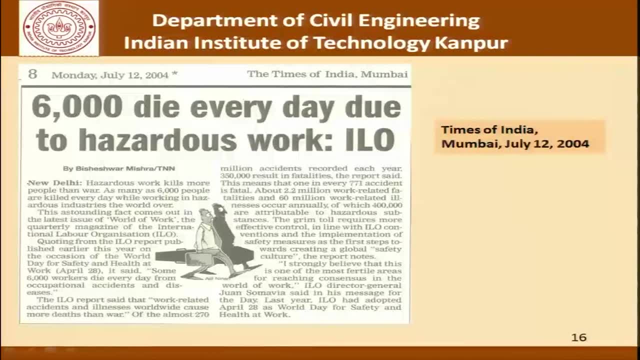 and so on. Now, this picture here is just a snapshot taken from the Times of India of 2004, and it says that 6000 people die every year due to hazardous waste. Now, when it comes to these numbers, we have to remember: these are statistics, the numbers. 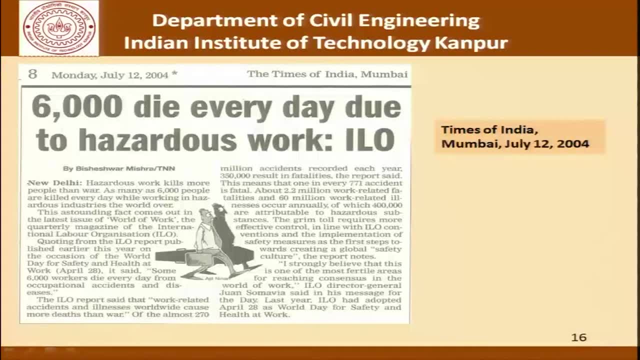 which have been collected by agencies from different countries and put together. So there could be a few things here and there: The exact definition as to what is hazardous work, what are the standards that are prevailing in different countries, whether the death occurs immediately after exposure to hazardous 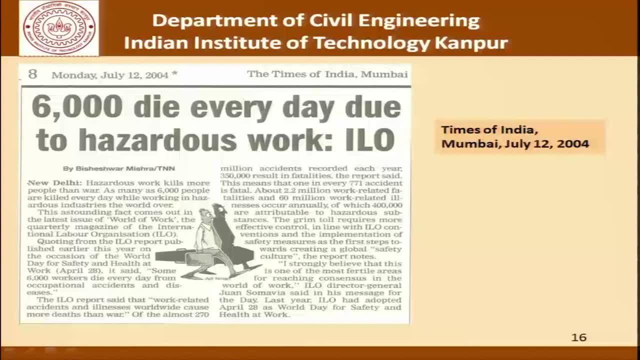 work. does this number include health related deaths, which are also, of course, occupational, occupational health related issues, or is it only accident related deaths? those details are the fine print, But the spirit of the discussion is that, indeed, occupational health and safety is a very, very 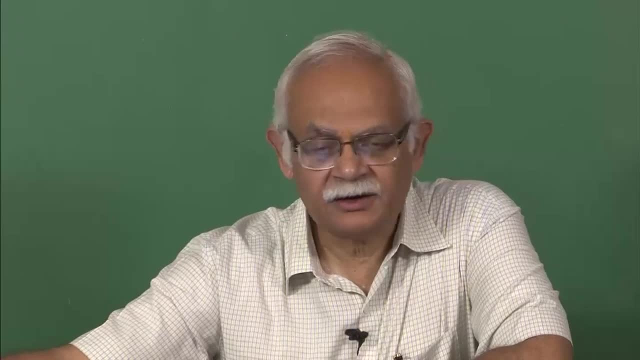 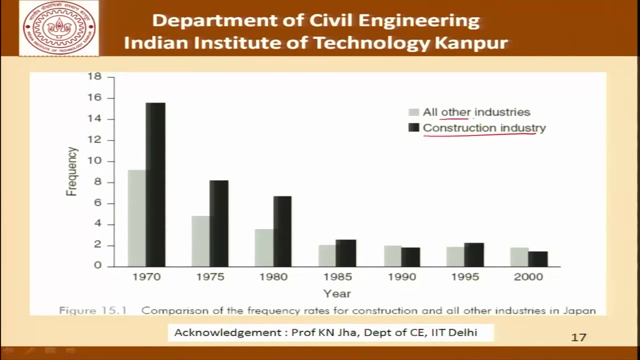 serious concern to the engineering profession, and that is why we are talking about it here. This picture here shows how the construction industry fares with respect to other industries, and these statistics are a little old. they are dated to about 2000 and are taken from 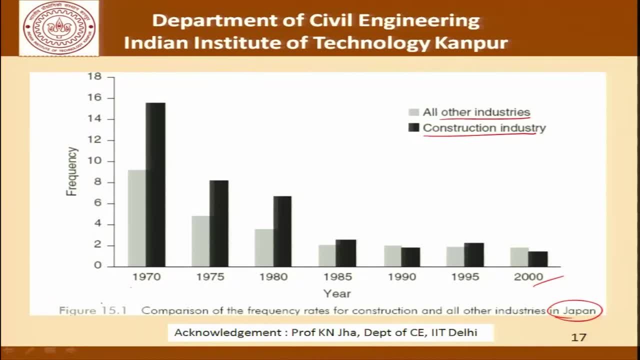 Japan. There are different ways of looking at this picture, and what I see is that, up to this point, here, the construction industry- the frequency of accidents was much higher than in the other industries. All these industries due to efforts which must have taken place around 1970, and so on. 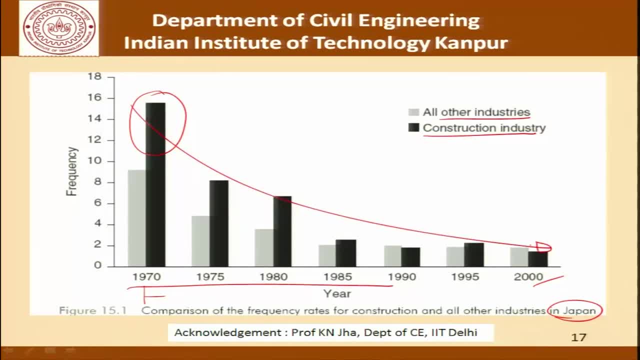 as far as the frequency is concerned, it has gone down. What can be stated is that in Japan, due to whatever sustained efforts that were taken to introduce safety measures at sites, introduce safety measures in the industry, tighten the safety culture and so on, there is a decline in the accidents. 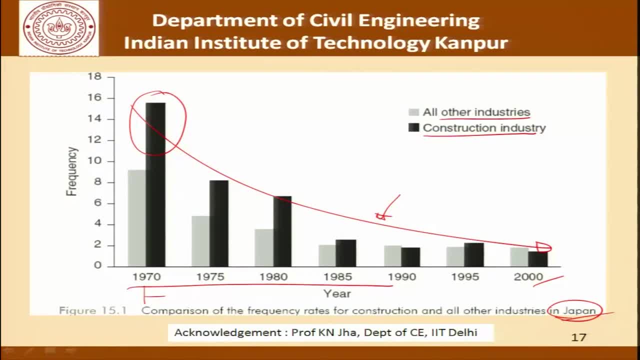 What is equally important to understand is that in the 70's, 75,, 80 and 85 and so on, the construction accidents frequency was higher than the other industries. that in 2000 has finally come to a situation where the construction industry frequency is lower than the other. 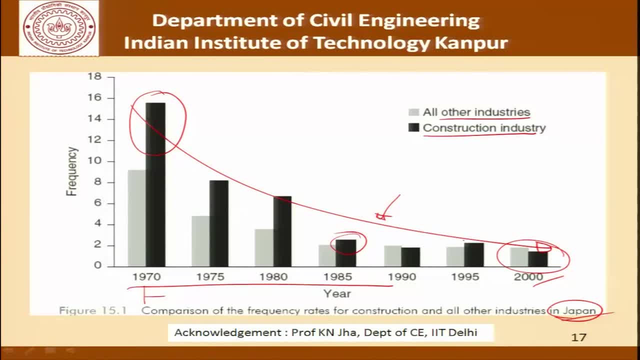 industry that the construction industry indeed put in a lot of effort to reduce the construction accident, to bring down the accident rate or the frequency as far as construction sites is concerned. So this is the kind of information that is very encouraging to see and I am sure there. 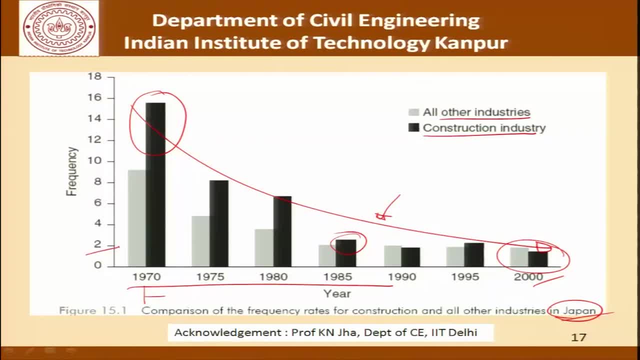 is a lot more to do. Please see that the number here is only 2.. So there is about 2 to 4.. This is the kind of number of accidents that we are talking about. I would like to invite you to go to the newspapers and any other source of information and try. 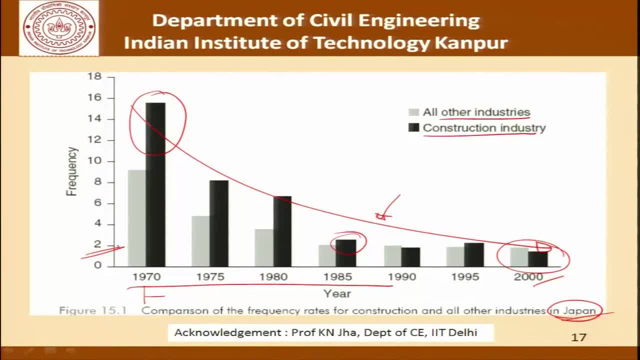 to find out what is the kind of numbers of accidents that are taking place around you, in the neighborhood. It could be the city, it could be the state, it could be the country. We are all in India, most of us- and it could be anywhere else in the world. 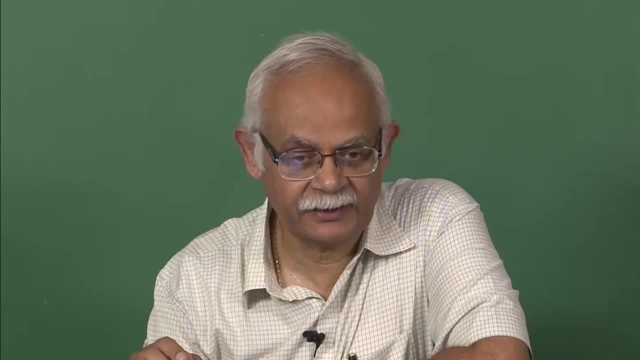 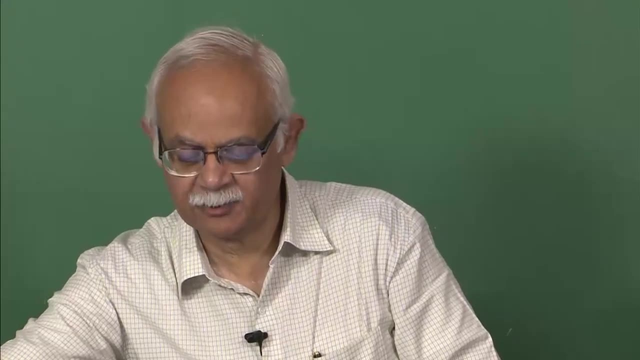 But please remember that this data is not easy to come by. There are lots of reasons for it and we are not getting into details of that, But, yes, a sustained effort can still be made and must be made. This is a study from the United States and UK, and this data is even more dated. 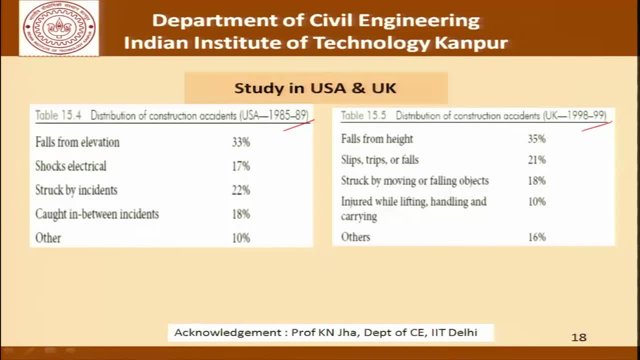 It is 89,, 98,, 99 and this gives us what is the breakup of the nature or the cause of construction accidents in United States and UK. We find that falls from elevation shocks struck by incident, that is, you are hit by 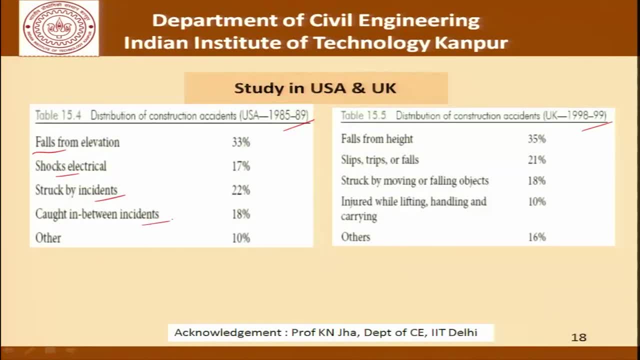 something caught in between accidents, meaning that you are caught between two objects and others. This is the breakup as far as the United States is concerned. So we find that fall from a height contributes to 33%, or one-third of the total accidents. 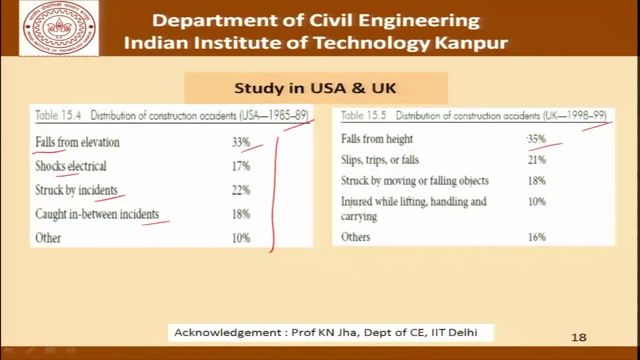 Fall from height in the UK in a different time period is about 35%. Trips, slips and falls is another 21, struck by moving and falling objects is 18,. injury by lifting, handling and carrying is 10 and the others is 16.. 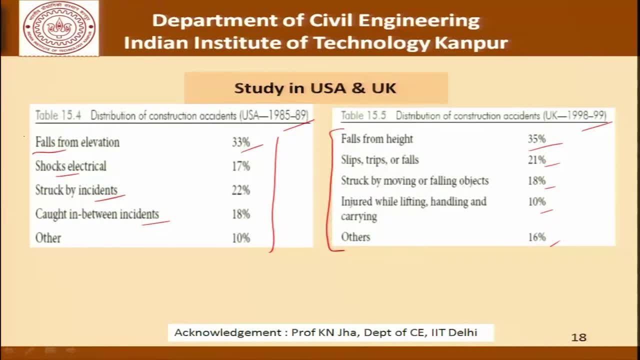 So it is not a matter of how we divide this. The issue is how we divide this. The issue really is to understand that there are different factors that contribute to an accident. We have to be careful about things which cause an accident. This is the information that we have about the Indian construction industry, ranging from 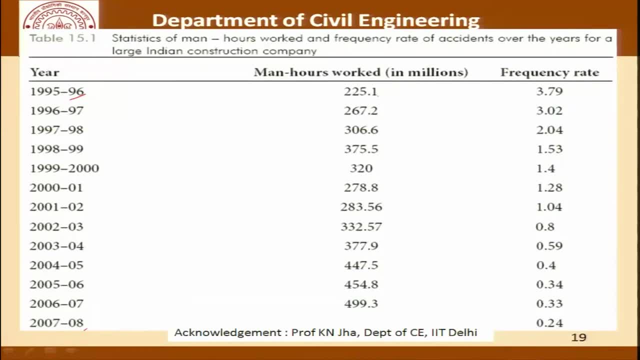 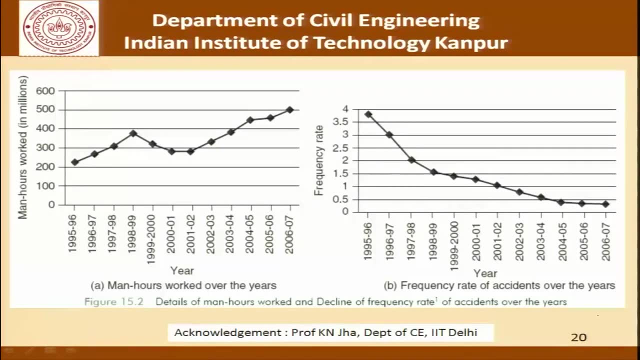 1995 to about 2008.. This is the million man hours being worked as far as the construction industry is concerned and this is the frequency rate. This picture here shows the man hours worked in millions and also the frequency rate. It is the same data that we saw earlier. 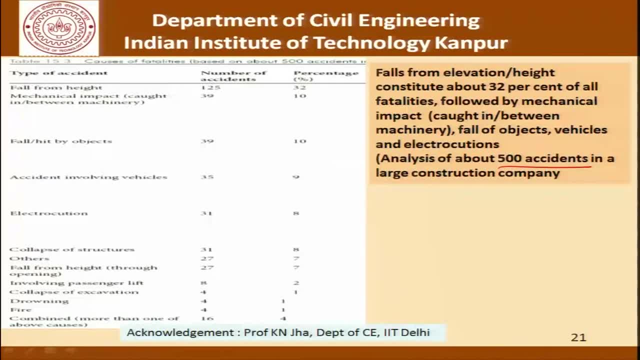 Now this picture is an analysis. Now what is the frequency rate of about 500 accidents? and here in India we find that fall from heights again contributes about 32%. Mechanical impact which is caught in between the machinery is 10%. Fall or hit by objects is another 10.. 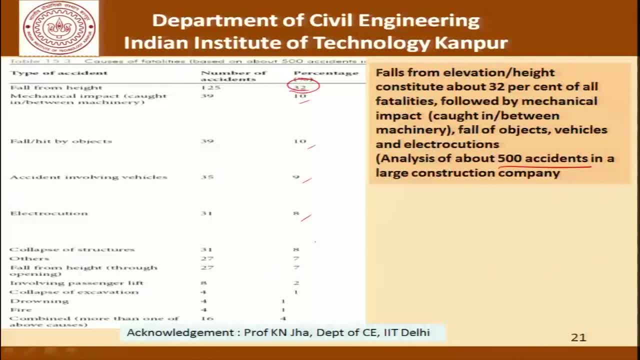 Accidents involving vehicles is 9.. Electrocution is 8, and so on. the list goes. So it is interesting to see that, no matter what, the fall from heights is about one-third of the total accidents. Now it is interesting also to see that when we say fall from heights, 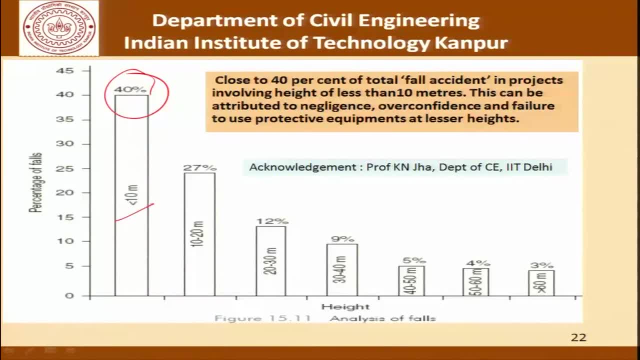 40% of the accidents are taking place at heights less than 10 meters. Now, this is a very interesting thing to look at, because when we say heights, there are two ways of looking at this discussion. One is: heights may mean high rise structures or towers where the worker is working at an 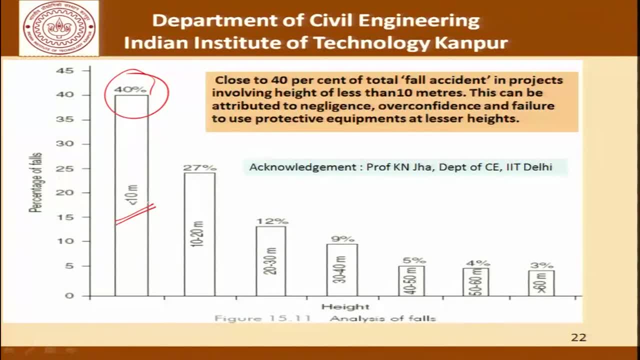 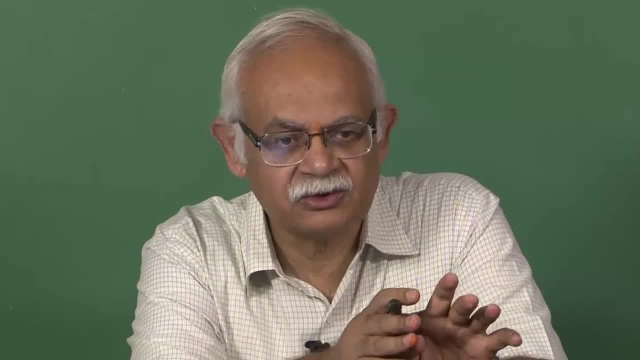 elevation, which is fairly high: 60 meters, 70 meters and so on. What we find in this statistic is that it is just 10 meters. 10 meters is about two to three-story kind of a building. From that height we have 40% accidents. 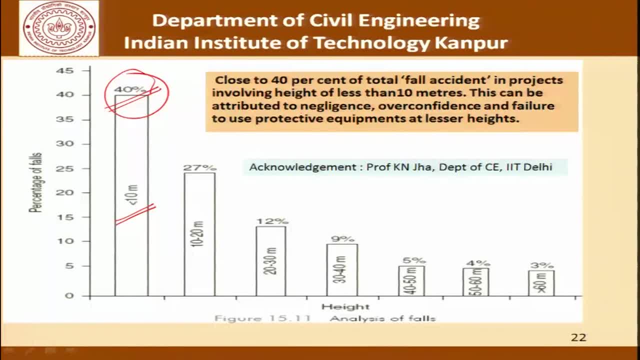 Now that is something which is very difficult to digest, because it shows negligence, overconfidence and failure to use protective equipment at lower heights. What happens is that workers, and perhaps the management, become complacent when the height involved is not very high. We allow, we compromise on the standards which are required for high-rise buildings. 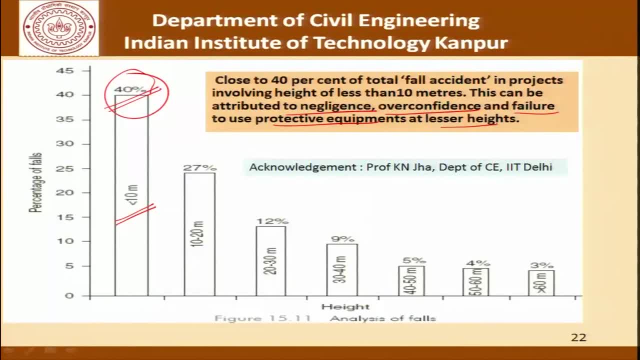 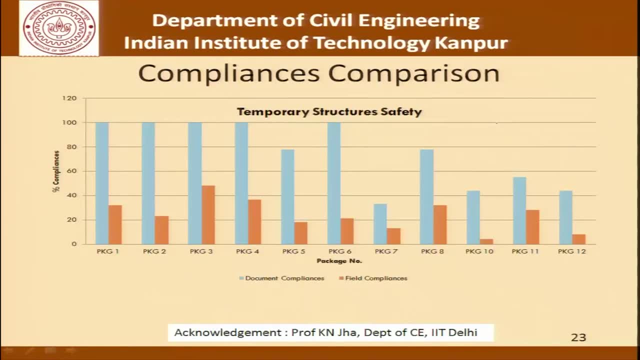 Working on heights, not realizing that an accident is an accident and it can happen at any height Moving forward. this is the compliance comparison which Professor Jha put together with temporary structures. There is something very interesting called document compliance and field compliance. Now what we find is that the document compliance is very high in a lot of cases. 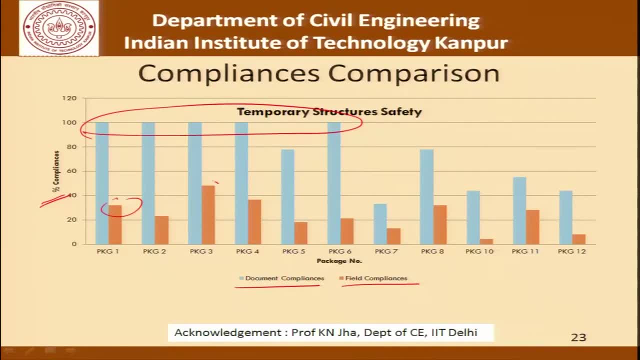 It could be as high as 100%, but the field compliance is very low. Now, this is something which is another very, very complicated. Thank you, Unfortunately, it is something which needs attention. The document compliance is high, but the field compliance is low. 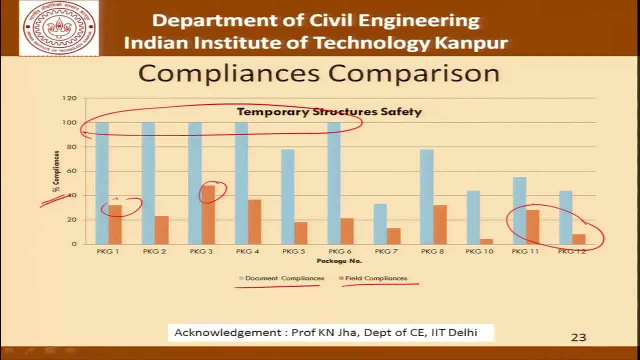 And this kind of data is very, very difficult obviously to get, but there has to be some basis to be able to draw this information. We cannot obviously share that kind of discussion with you, but please remember and appreciate the fact that it is important that the field practices what is laid down in the document. 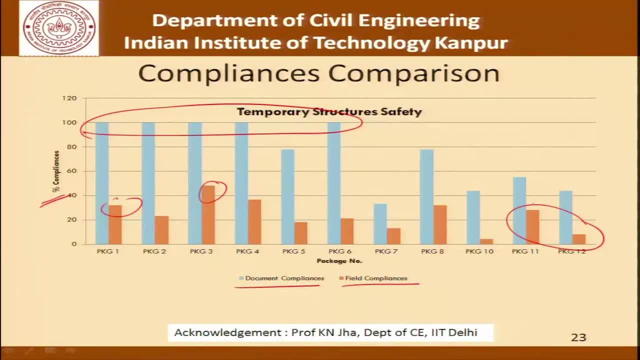 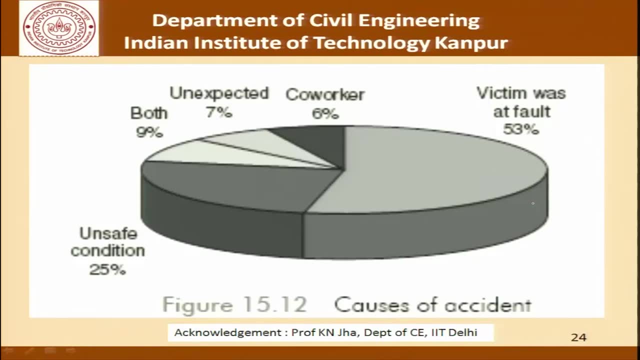 Unless that is done, it is very difficult to ensure construction safety. Moving forward, as far as cause of accidents is concerned, here we are introducing a few other things. We are saying that the victim was at fault is 53 percent- There were some unsafe conditions- which is 25 percent. one-fourth, 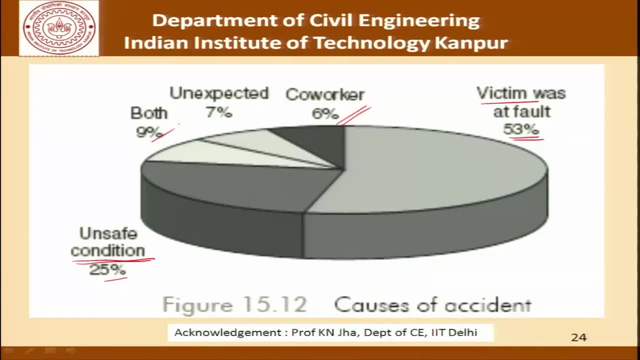 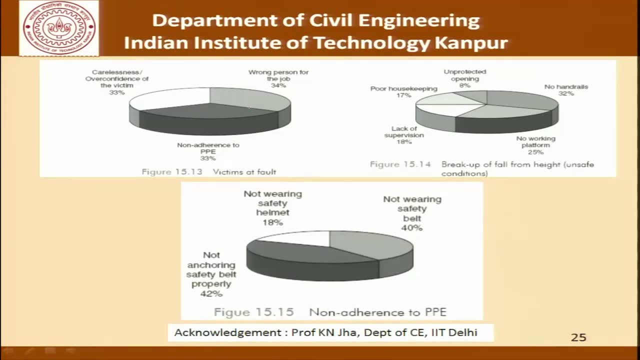 The co-worker was at fault. that is about 6 percent. Both were at fault is 9 percent and unexpected is 7 percent. Let us try to look at a few other pie charts like this: No handrails is 38 percent. 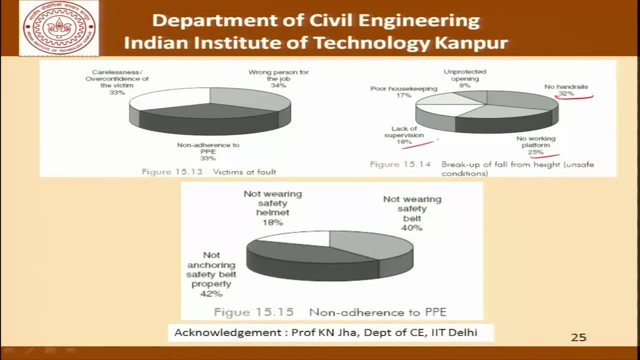 32 percent. No working platform: 25 percent. Lack of supervision: 18. Poor housekeeping: 17. And unprotected opening is 8.. This is the breakup of fall from height When we look at the fault of the victim: non-adherence to PPE, which is the personal protective equipment. 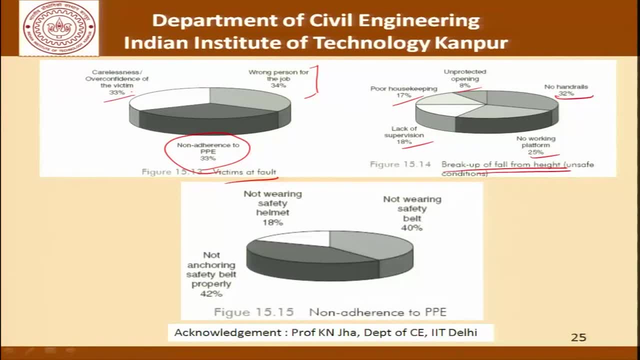 wrong person for the job is 34, and carelessness, overconfidence of the victim is 33.. So very nicely, one-third, one-third. It really shows that it is a matter of compliance. It is a matter of educating the worker to use the kind of equipment to follow the kind. 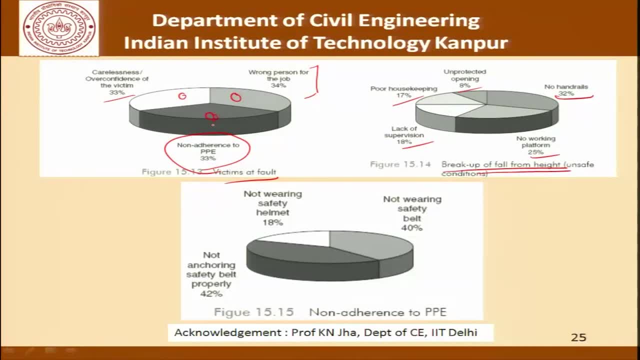 of norms which will make the construction site a safe place to work. As far as non-adherence to PPE is concerned, safety belts is 40 percent, helmet is 18 percent and not anchoring the safety belt properly is 42 percent. 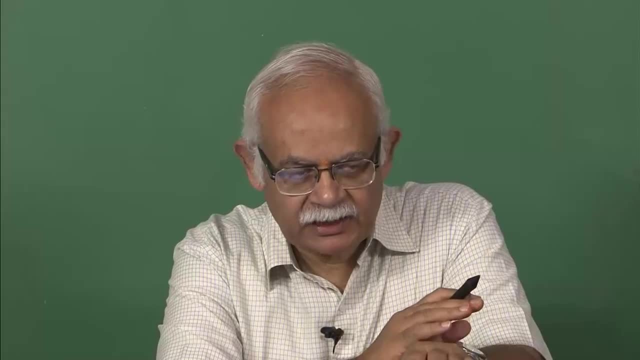 So some of these things we will talk again when it comes to non-adherence to PPE, All right, to details of PPE and so on, But at this point in time, when we are trying to talk about the different issues which are, 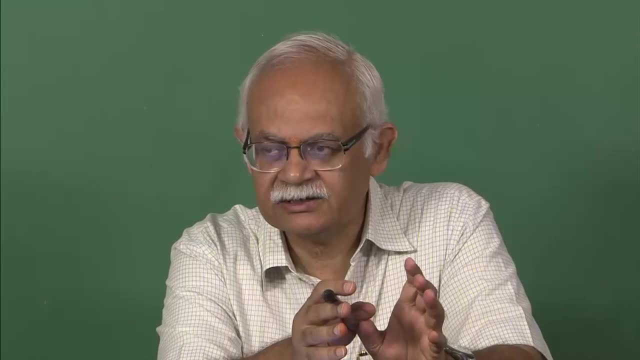 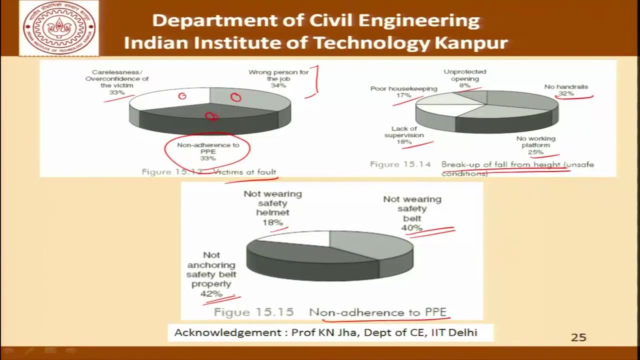 related to construction safety. it is enough to understand that there is a whole lot of education that needs to be imparted. There is a whole lot of analysis of data which has to be done in order that construction managers understand the importance of safety, know where to concentrate as far as steps. 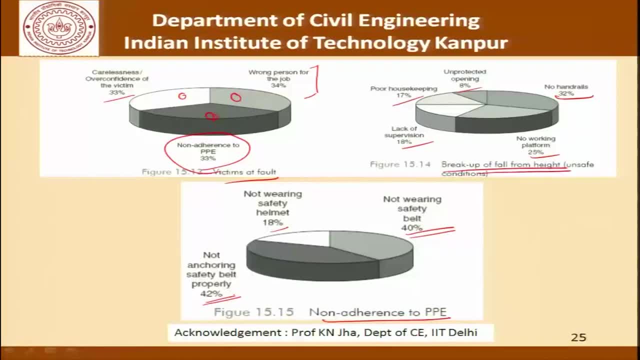 to reduce construction accidents are concerned. From this picture and the previous one, there is also a very important conclusion that we can draw. Let me leave that question to you: What percentage of these accidents do you think are preventable? What is the percentage of accidents which would not have happened if there was proper? 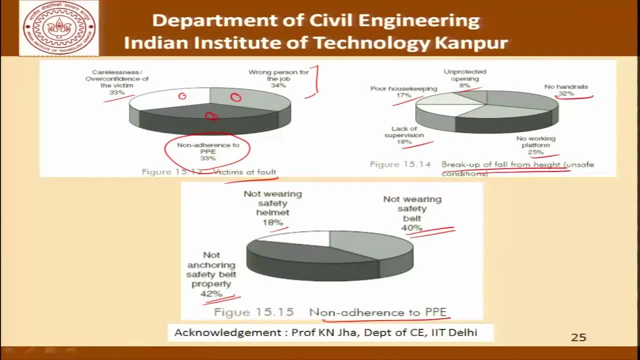 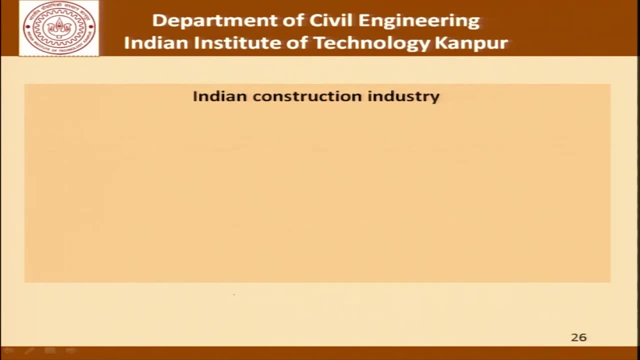 education and proper compliance of provisions. We will answer this question at a later point in time in this discussion, But for the time being, just keep it at the back of your mind. This slide tells you about the Indian construction industry. There are 200 large firms, including large public sector construction undertakings, 90,000. 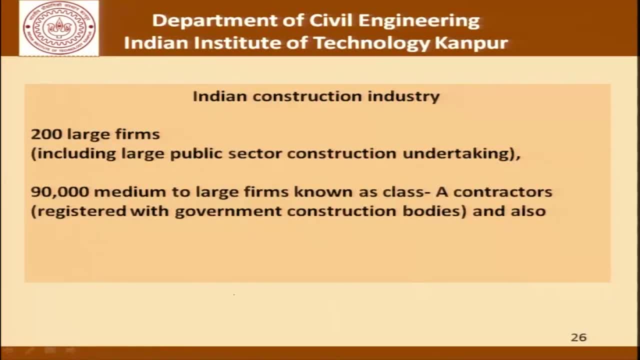 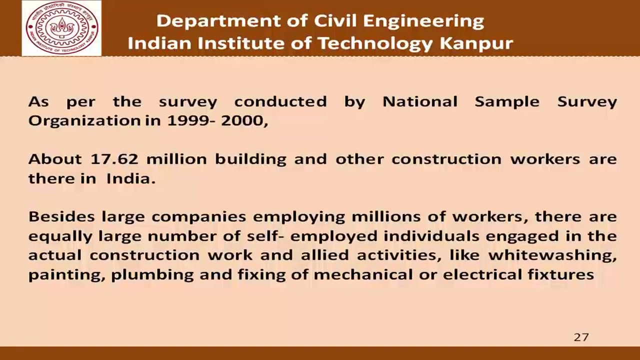 medium to large firms, known as class A contractors, registered with government construction bodies, and there are 6 lakh, that is, 600,000 small firms or contractors and subcontractors who execute small jobs, including repair. Now, the idea of showing you these numbers Is to basically make you aware of the challenges involved when it comes to implementing construction. 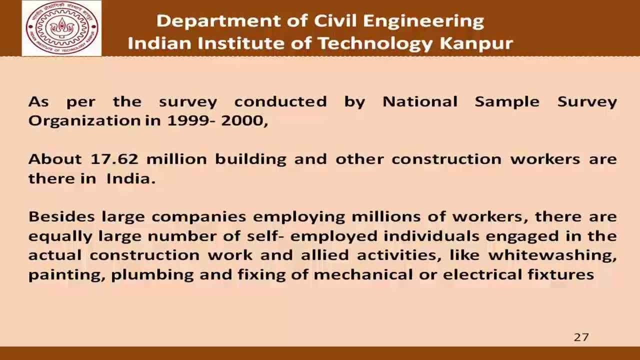 safety laws or construction safety rules. Now, as per a survey conducted by the National Sample Survey Organization in 2000,, about 17.62 million building and other construction workers are working in India at different construction sites, And besides large companies employing millions of workers, there is an equally large number. 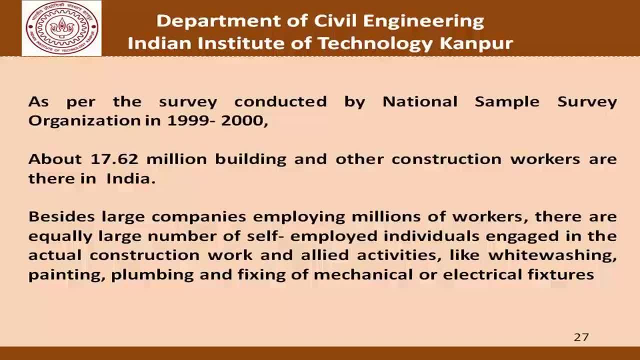 of self-employed individuals engaged in actual construction. What are the challenges? Well, the first challenge is that the construction industry is a very large employer of people in the country, And that is true with a lot of developing countries where infrastructure is being built. 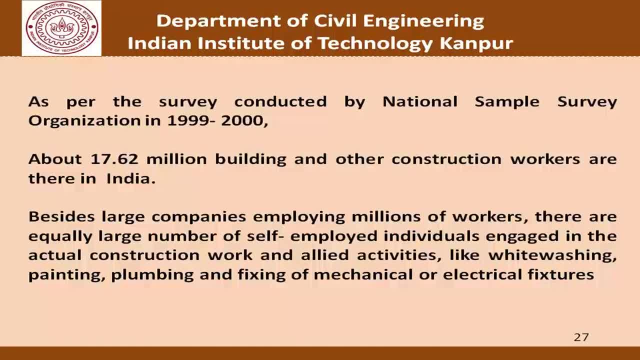 So the construction industry, by nature, is sometimes a labor intensive industry and that is very important to appreciate and understand and keep at the back of your mind when we talk of provisions relating to industry, Industrial safety or construction safety as far as that diverse group of workers is. 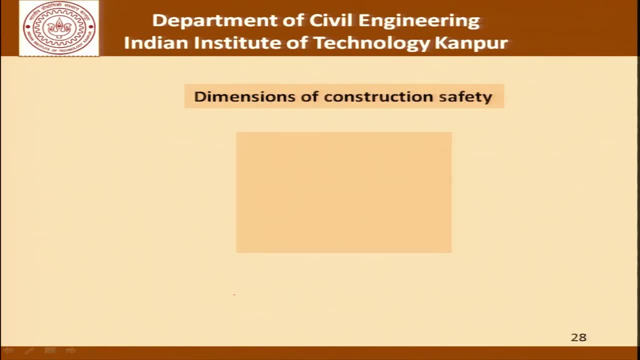 concerned. Now, before we go further, let us talk of the different dimensions of construction safety studies. Cost, of course, accidents- there is a cost involved. we will talk about that in a subsequent lecture. It is a direct cost, indirect cost, direct cost to the company, direct cost to the worker. 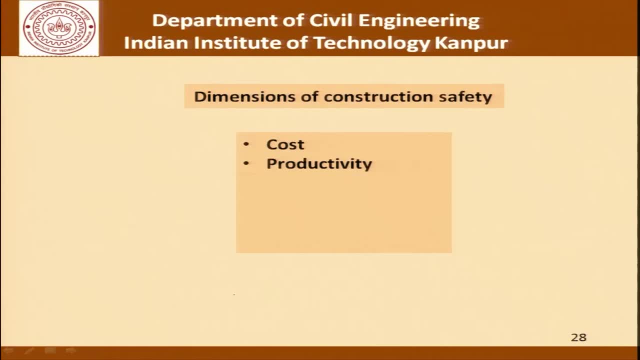 indirect cost to both of them, and so on Loss and productivity. the site is closed, the debris has to be removed and only then construction work can start. So there are delays, there is a loss on productivity, human suffering, injuries, deaths, disabilities. 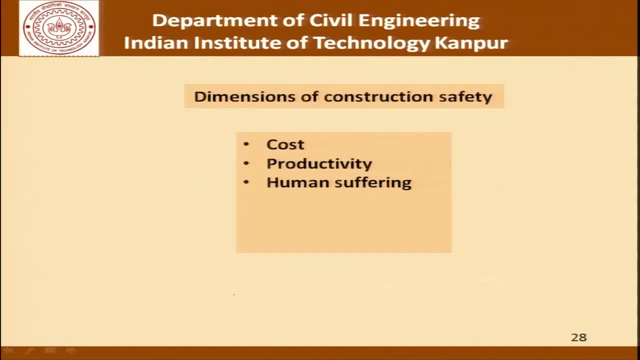 temporary, permanent hospitalization, not only for the worker or the victim, but also their families and near ones. it is a very, very difficult and a painful situation. statutory problems Including issues such as being barred from future contracts, the impact of accidents. 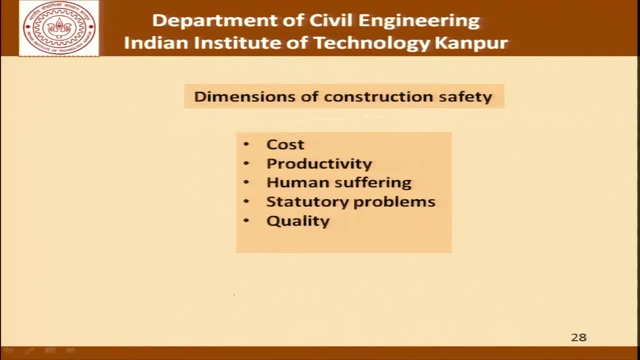 on quality. quality and safety are very closely related to each other and I am leaving it to you to think about this relationship, how it exists and why it exists, and the loss of reputation to the construction company. These are some of the dimensions of construction safety which must be kept in mind by the safety. 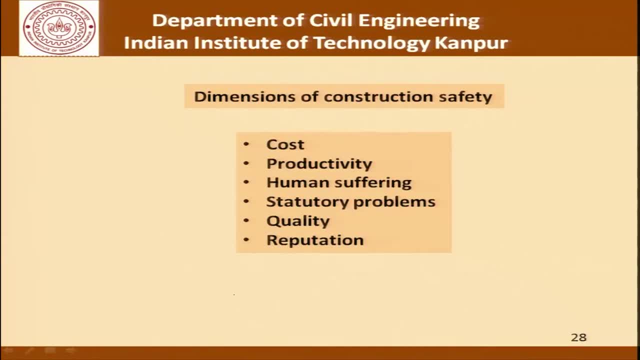 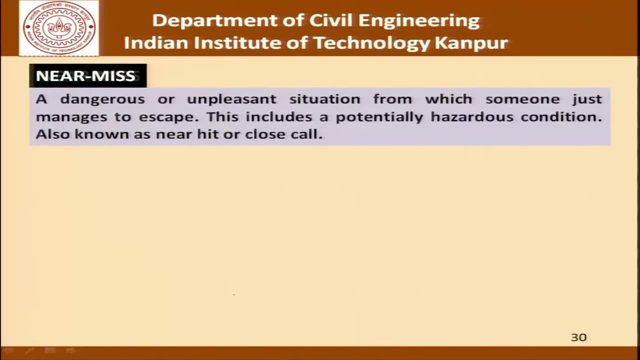 organization or the companies engaged in construction work. Now let us briefly look at some of the terms used in construction safety. The first thing is a near miss. it is a dangerous and an unpleasant situation from which someone just manages to escape. This includes a potentially hazardous condition and is called a near hit or a close call. 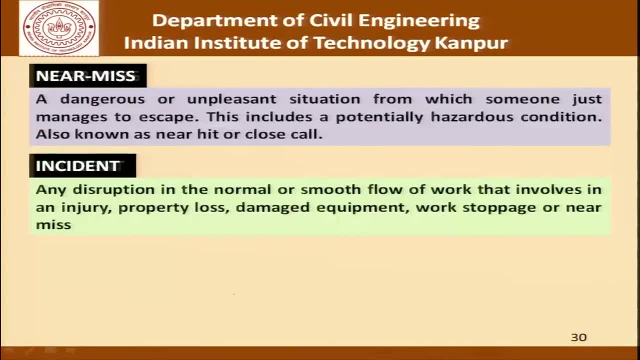 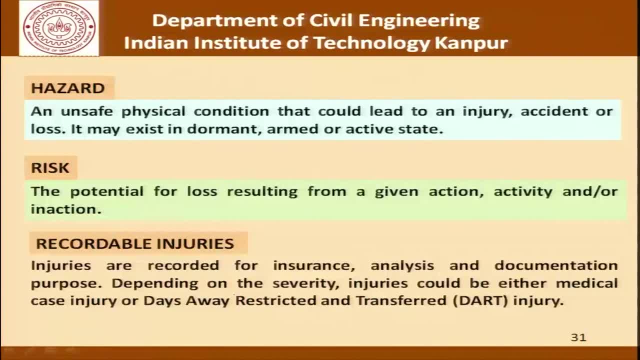 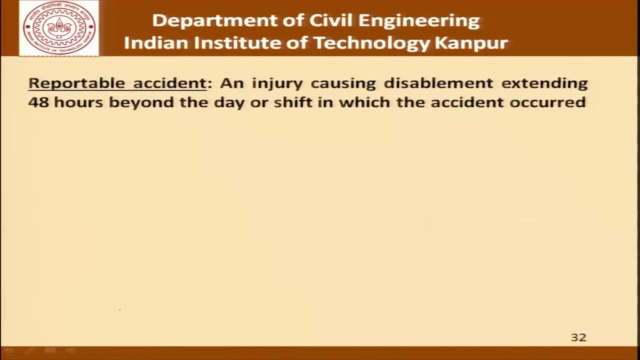 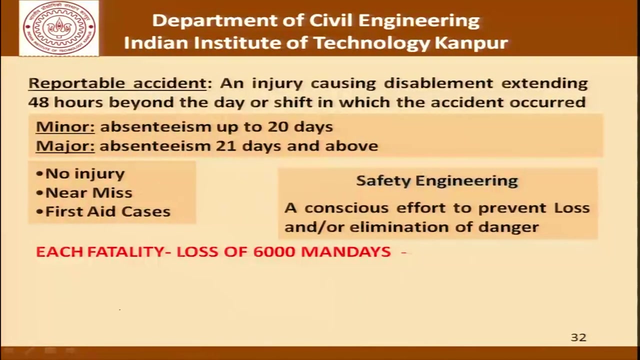 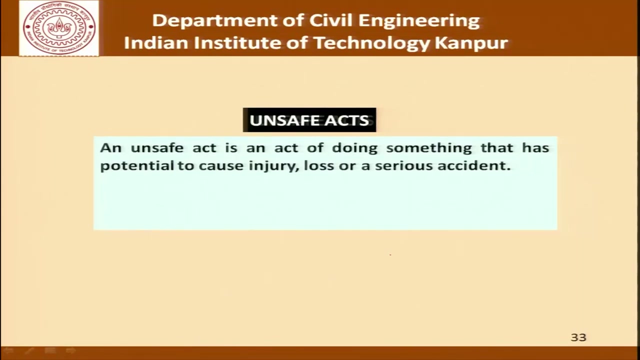 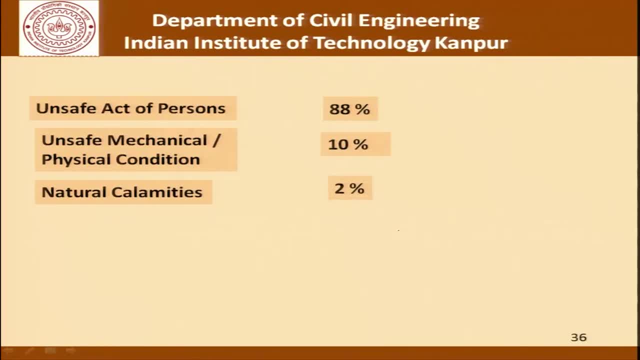 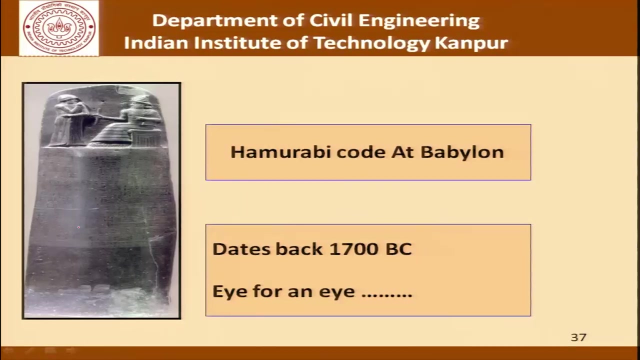 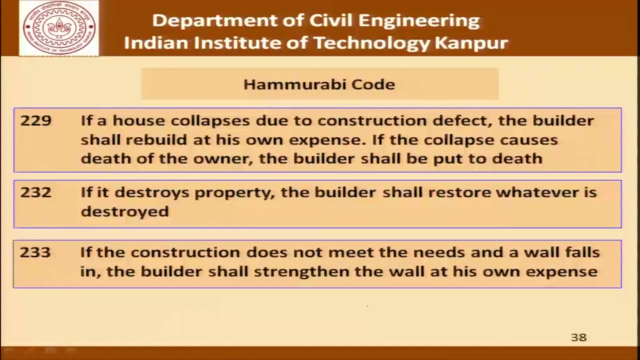 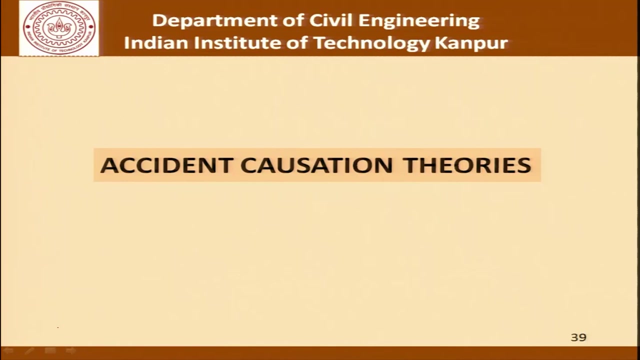 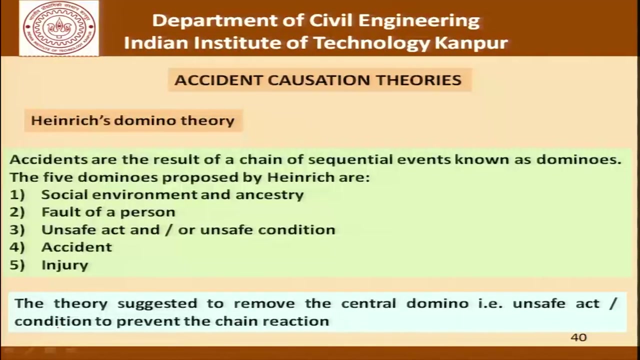 Heinrich, whose domino theory says that accidents are the result of a chain of sequential events. 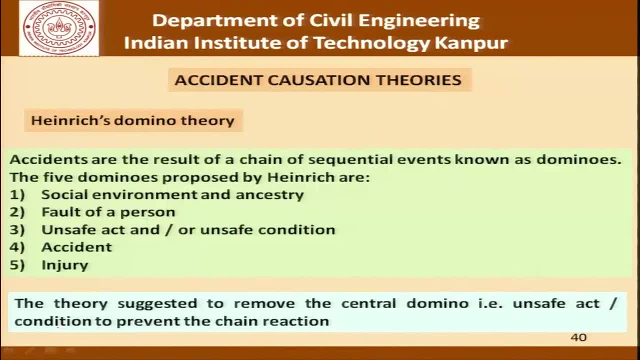 known as dominoes, And the five dominoes proposed by Heinrich are: social, environment and ancestry, fault of a person, unsafe act and or unsafe condition, accident and injury. And the theory suggests to remove the central domino. unsafe act to prevent the chain of. 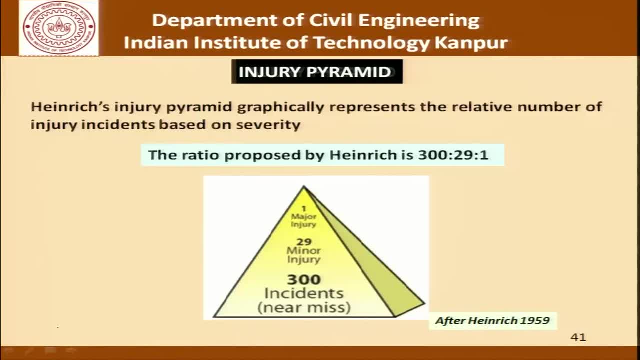 accidents. There is a very interesting injury pyramid proposed by Heinrich, which says that for 300 near misses or incidents, only 29 would have minor injuries and one major injury. Basically, what it says is that only one major injury will happen in 330 reportable accidents. 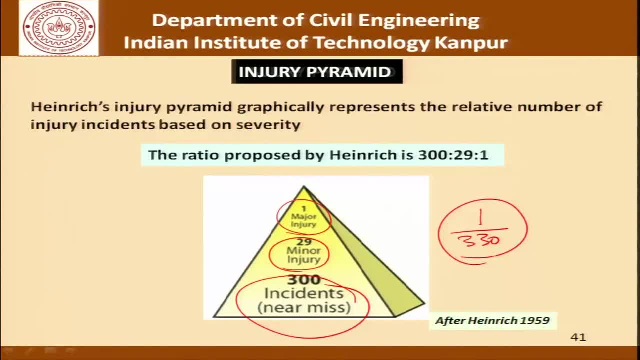 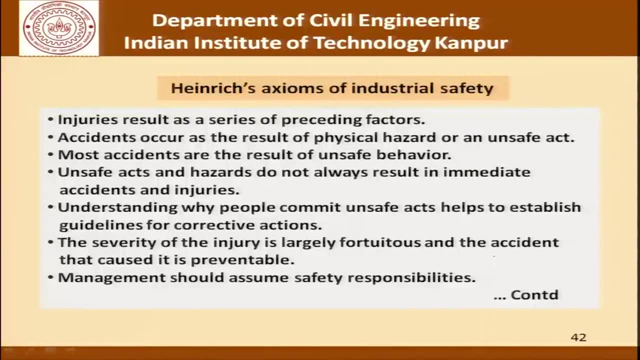 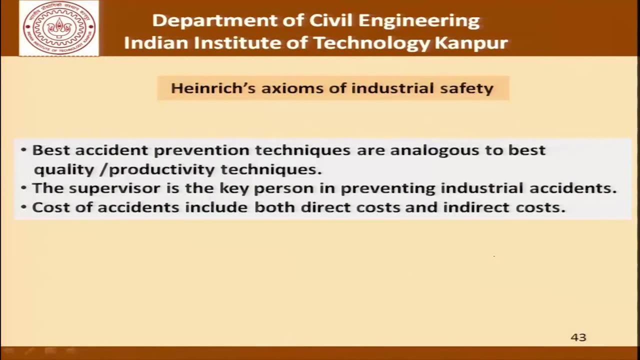 But that itself is cause enough for us to take steps and prevent accidents. These axioms from Heinrich on industrial safety, I am leaving it to you to read, because they are often focused on industrial environment, which is slightly different from construction safety. And best accident prevention techniques are analogous to best quality and productivity. 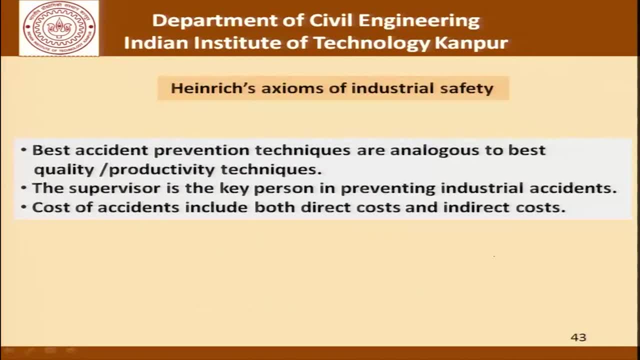 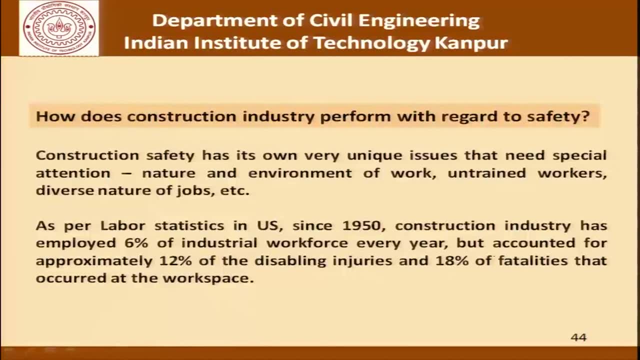 techniques and the supervisor is the key person in preventing industrial accidents, and the cost of accidents include both direct and indirect costs. We have already gone through this discussion a little bit earlier as to how the construction industry performs with respect to safety. The construction safety has its own very unique issues that need special attention. that nature 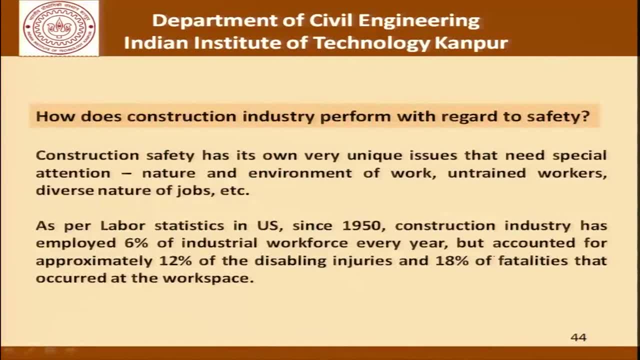 and environment of work, untrained workers, diverse nature of jobs- we have already talked about. We discussed this at the outset of the discussion today and, as per labor statistics, in the United States, since 1950, construction industry has employed 6 percent of the industrial workforce. 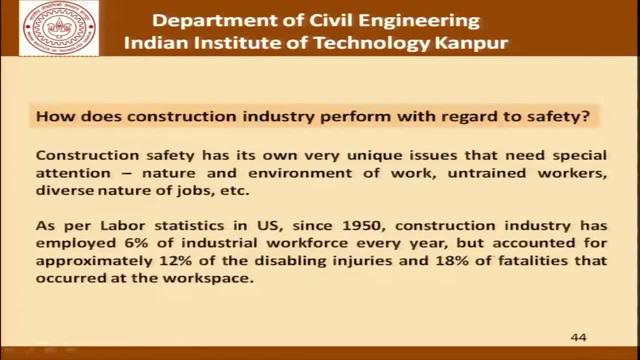 every year, but has accounted for 12 percent of the disabling injuries and 18 percent of the fatalities that have occurred at the work place. This is exactly the kind of statistics which we had shown for Japan, where the information was available over the period of time, that, yes, there was a time when construction industry 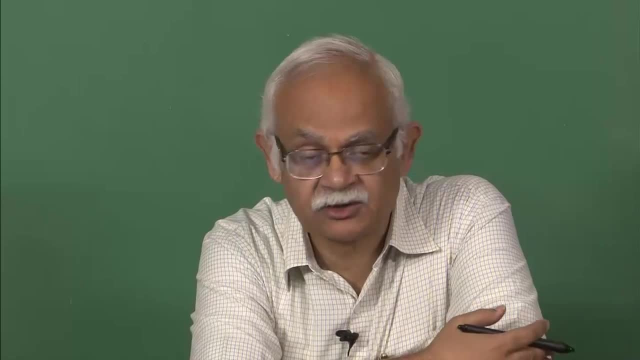 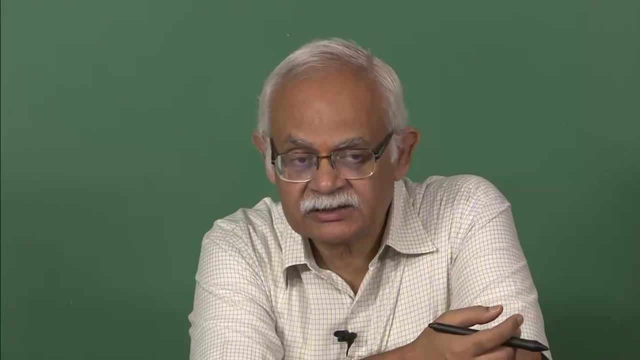 was having a higher frequency of accidents. Of course, in this case, it is talking about fatalities. It had a higher accident rate and therefore possibly a higher fatality rate, but that has come down over a period of time. As far as the United States is concerned, this data is something which you need to do as 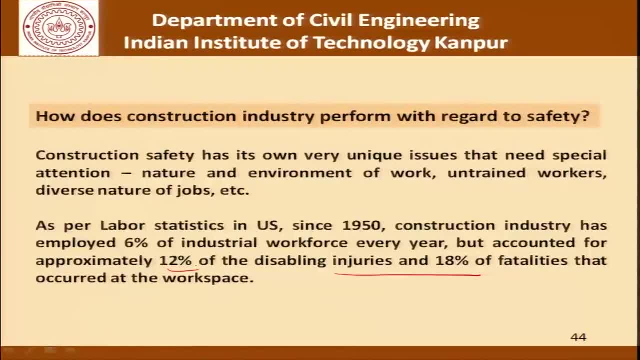 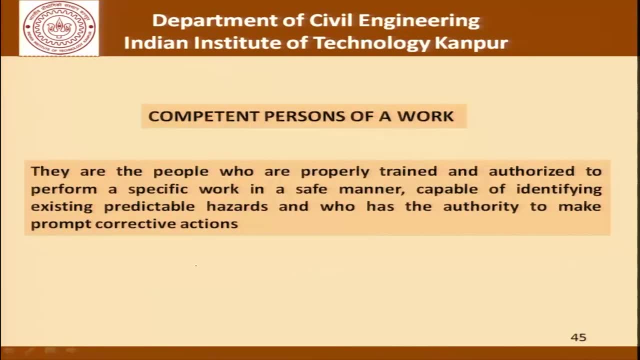 an exercise if you are interested in this subject and get it better understanding. Now, one important thing that we must understand as far as construction safety is concerned, that competent persons are very, very important to be identified for the construction industry. We have to understand that the construction industry is a very important part of the construction. 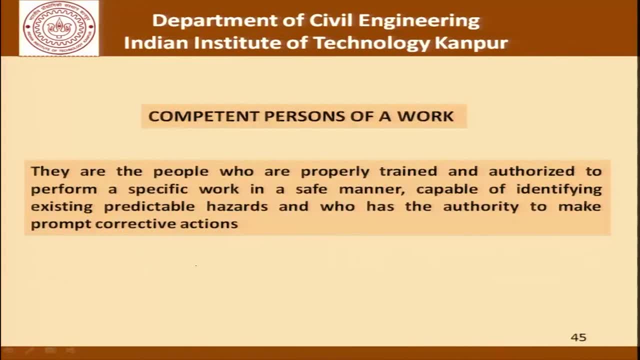 industry. We have to understand that the construction industry is a very important part of the construction industry. There are people who are properly trained and authorized to perform a specific work in a safe manner, capable of identifying existing predictable hazards, and who have the authority to make prompt corrective actions. 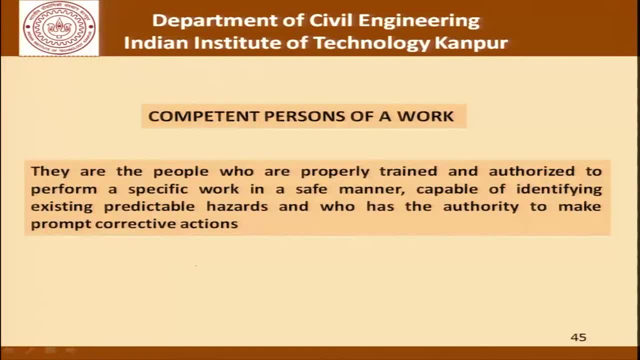 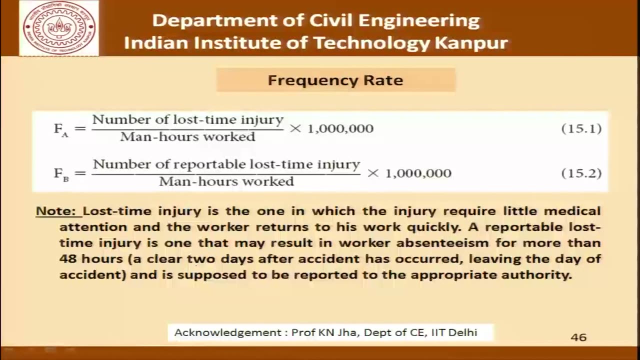 It's very important that people at construction sites do not try to do others work. It's very important that they understand the issues involved with training and handling different environments and different works, even though they may look simple, It's important for us to understand some definitions of different statistical parameters. 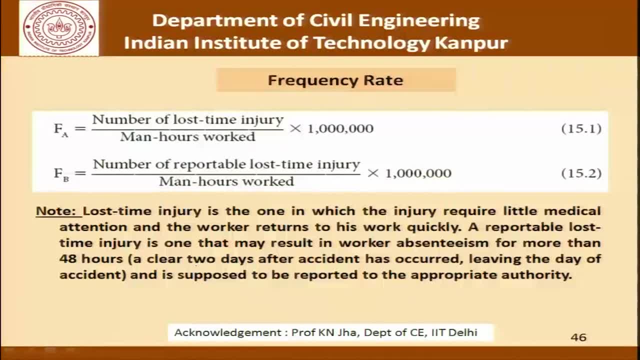 which are used or can be used to compute the kind of statistics that we have been talking about: frequency rate, reportable accidents, fatalities and so on. Now, obviously it's important that the man hours worked is something which has to be kept into, Obviously, the number of accidents. 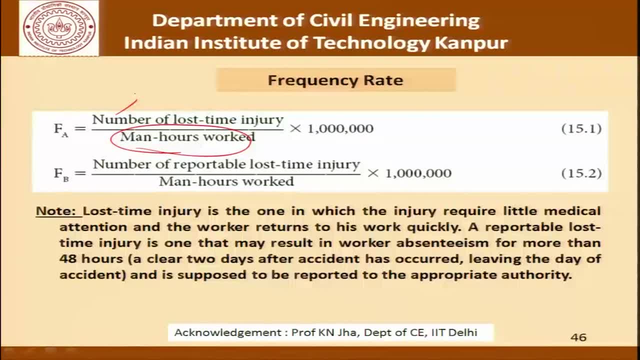 As an absolute number is one parameter, But those number of accidents have to be viewed in perspective with respect to the man hours that have been put in. So if we are not working at all, then obviously the chances of accidents are zero, But that doesn't mean that the frequency is zero. 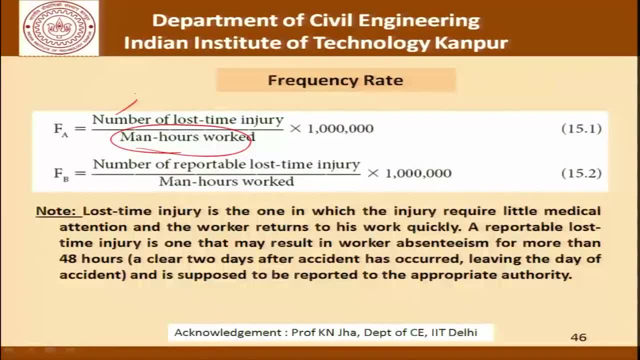 Only when there is a lot of work being done and man hours being put in. then we have to see whether a company is actually having a low frequency rate or not. So in this case we have man hours worked In the denominator and we have statistics like frequency F A and F B, which is number. 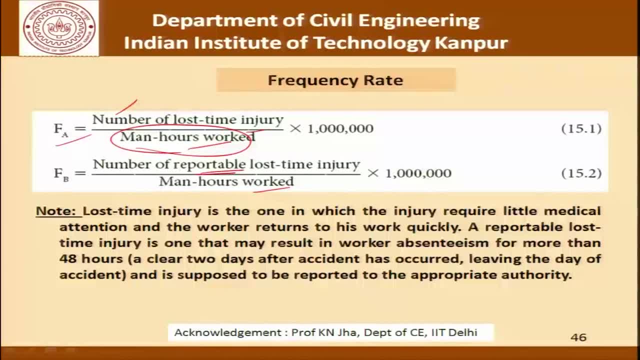 of reportable lost time injuries and number of lost time injuries total, which is given to us with respect to a million here. So because the man hours will give you a very large number, so it's multiplied by a million to get the numbers in a more reasonable range. 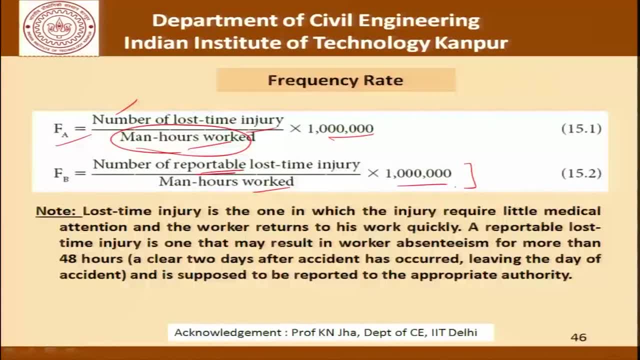 Lost time injury is one in which the injury requires little medical attention and the worker returns to his work quickly. A reportable lost time injury is one that may take the worker to be absent from his work for 48 hours, a clear two days after the accident has occurred, and leaving the day. 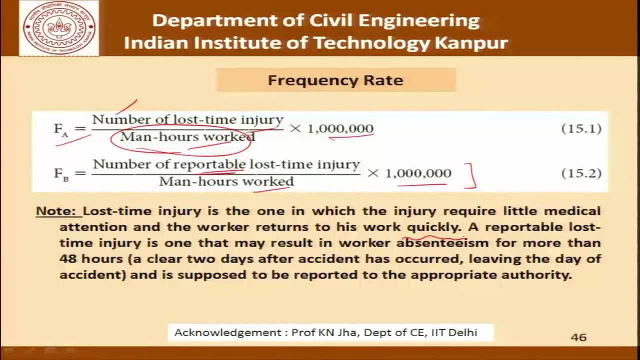 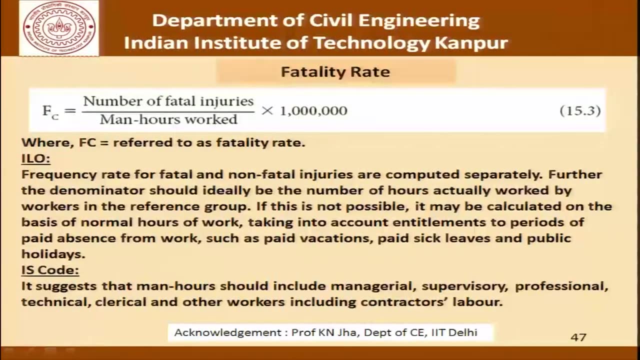 of the accident and is supposed to be reported to higher authorities. Now, of course, at different sites, with different clients, with different regulatory bodies, this appropriate authority could be different Fatality rate, similarly is the number of fatal injuries, Again with the man hours worked in the denominator. 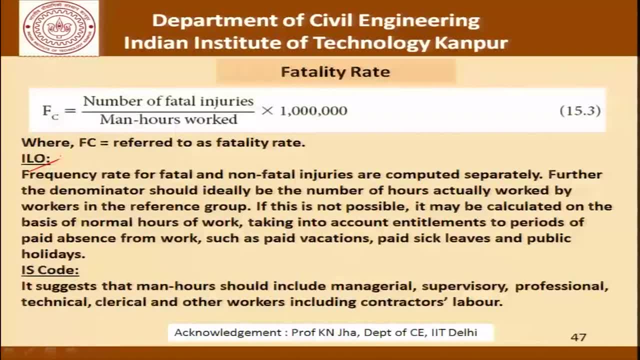 So, whereas the ILO suggests that the frequency rate for fatal and non-fatal injuries are computed separately, and the denominator should ideally be the number of hours actually worked by the workers in the reference group, and if this is not possible, it may be calculated on the basis of normal working hours, taking into account entitlements to periods of paid. 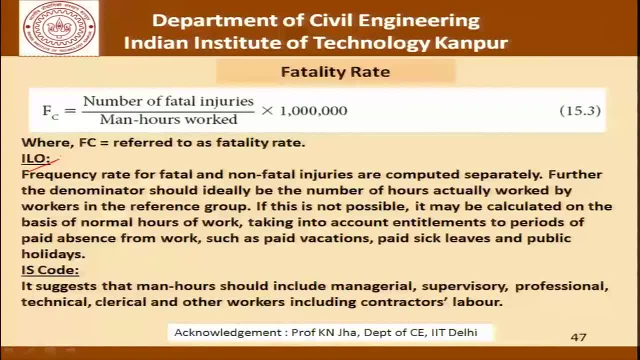 absence from work, such as paid vacations, paid sick leaves and public holidays. Similarly, When courts are concerned, they suggest that man hours should include managerial, supervisory, professional, technical, clerical and other workers, including contractors labours. So this is what gives you the idea that it is not simple to compute the man hours worked. 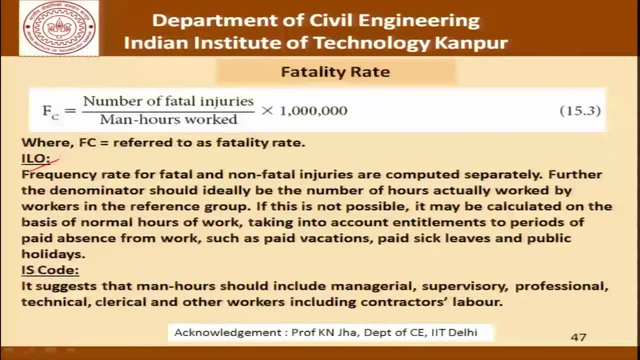 Whose man hours are we talking about? Are we talking about only the workers at site, or we are also including the workers who are working in offices supporting that site work? So it is not that one is right or the other is wrong. It is only a matter of having accountability. 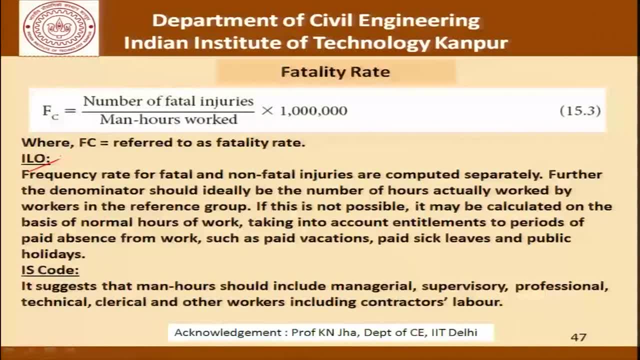 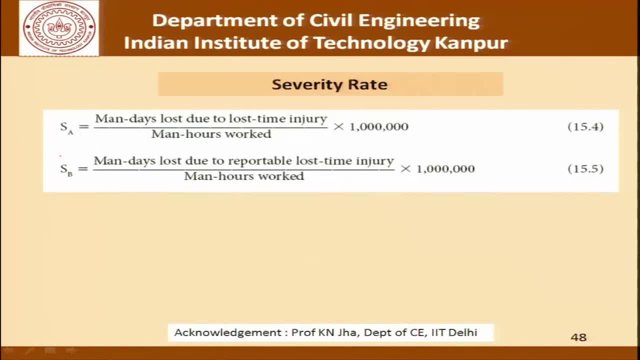 It is only a matter of having accountability, It is only a matter of having a clear definition which is understood by all concerned and is followed, as far as generating these statistics are concerned. Similarly, when it comes to severity rate, there is A and B, which is man days lost due to lost. 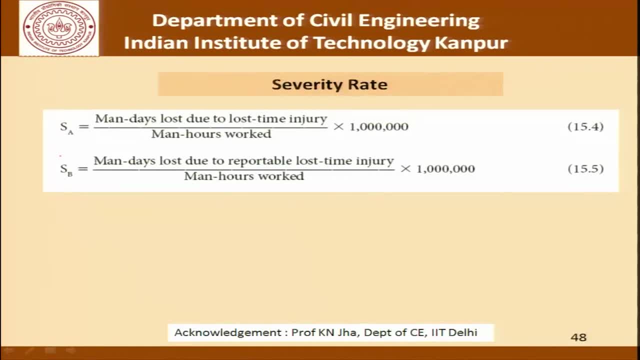 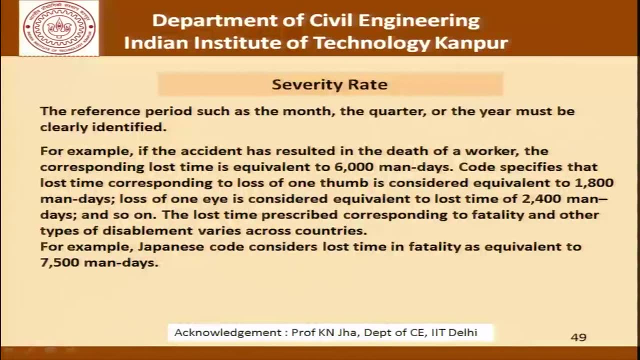 time injuries and man days lost due to reportable lost time injuries, again related to the man hours. As far as severity rate is concerned, the reference period, that is, the month, quarter or year, must also be clearly identified, For example, if an accident has resulted in the death of a worker. 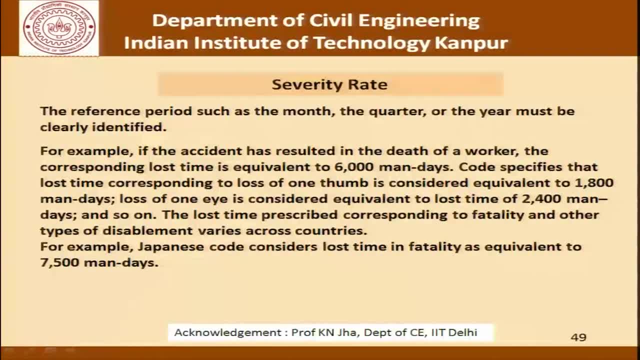 The corresponding lost time is equivalent to 6000 man days. We had mentioned this in the slide earlier, if you will recall- And the code specifies that the lost time corresponding to loss of one thumb is considered equivalent to 1800 man days. Loss of an eye is considered equivalent to lost time of 2400, and so on and so forth. 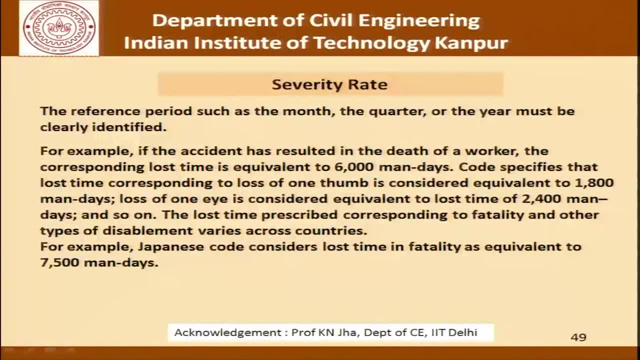 Construction accidents can have minor injuries, major injuries, which include temporary disability, maybe permanent disability, and all that has to be finally reduced to how much is the lost time? Now, that lost time is difficult to compute and therefore codes also lay down certain numbers, such as the number suggested here, in order to assign a certain amount of severity. 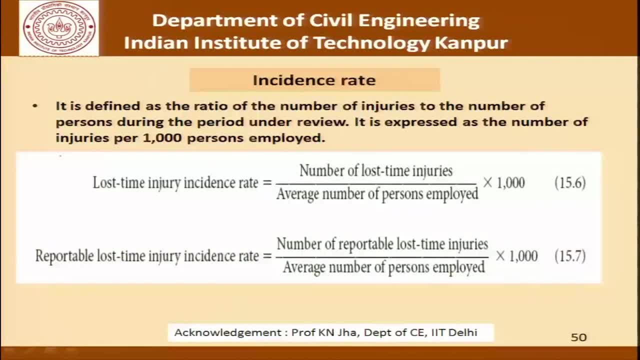 to a certain accident. Similarly, the incident rate is defined as the ratio of number of injuries to the number of persons during the work period under review and is expressed as a number of injuries per 1000 people employed. So here we have two clauses: the lost time injury incidence rate and the reportable lost. 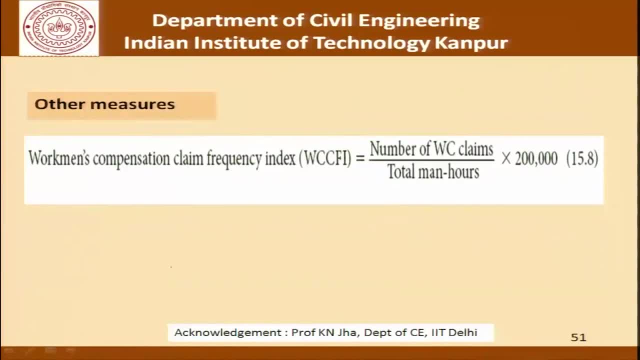 time injury incident rate, Which is defined as given here. and then, of course, there can be other measures which can be adopted to quantify the safety performance of a construction company. It could be workman's compensation claim frequency, which is the number of claims to the total. 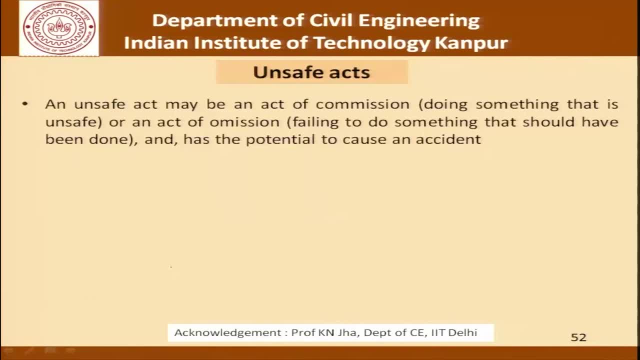 number of man hours worked. Let us come back to this discussion on unsafe acts and unsafe conditions. once again, An unsafe act may be one of omission, doing something that is unsafe, or an act of omission which is failing to do something which should have been done and has the potential to cause. 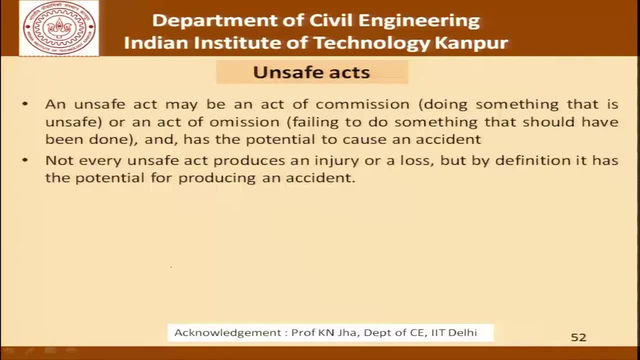 an accident. Not every unsafe act produces an injury or a loss, but by definition, it has the potential of producing an accident. A worker may commit unsafe acts regardless of the initial conditions of work, whether the condition was safe or unsafe. It could be on account of physical or mental deficiency, eyesight, hearing, fatigue. 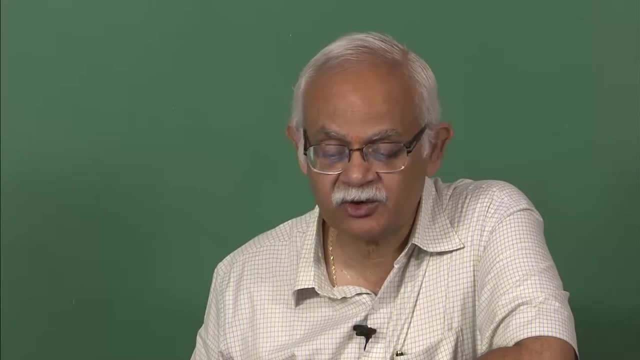 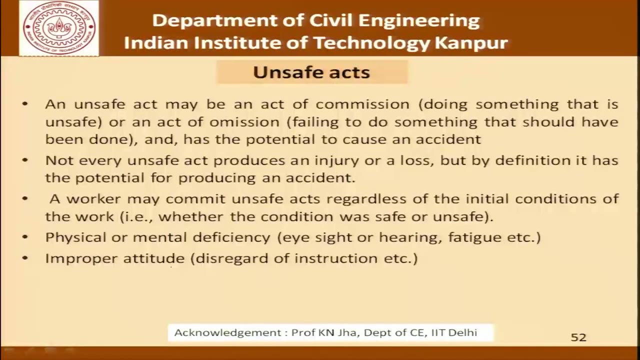 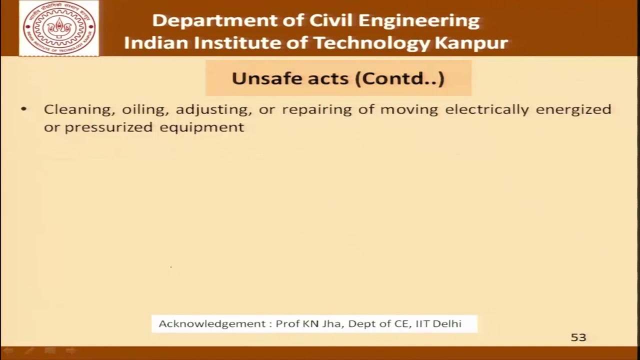 These are conditions which could induce or cause a worker to commit an unsafe act: Improper attitude, which is disregard of instruction. It could include overconfidence, arrogance and, if we continue with this list, cleaning, oiling or adjusting or repairing of moving electrically energized pressurized equipment. 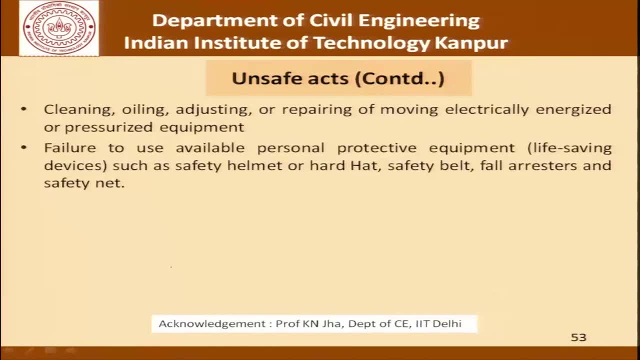 while they are running. Failure to use available personal protective equipment like life-saving devices such as helmets, hard hats, safety belts. Improper use of equipment which could include overloading. Improper use of hand or body parts Gripping objects insecurely. 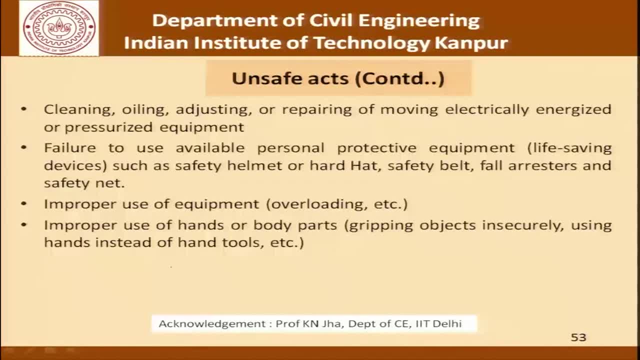 Using hands instead of hand tools. These are all things which are coming under the larger ambit of unsafe acts and obviously with the proper amount of worker training they can all be eliminated. Taking unsafe positions or postures: for example, it could be under suspended loads riding. 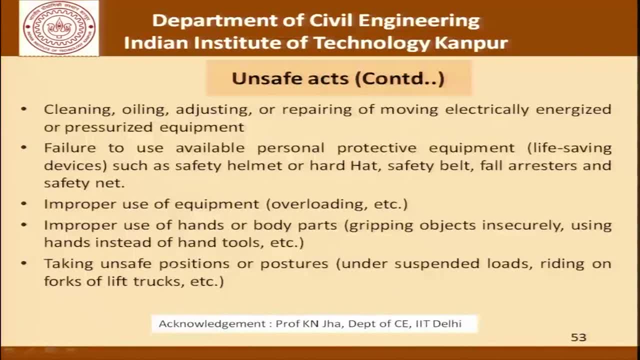 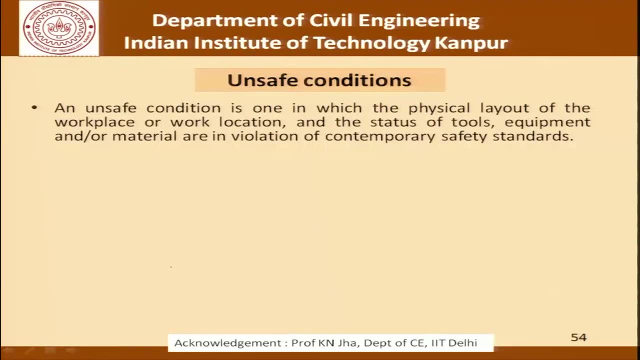 on the fork of lift trucks. Time permitting will probably go into some of these actual cases of accidents arising out of this kind of unsafe behavior. Now coming to unsafe conditions, That is, one when the physical layout of workplace or work location, the status of tools, 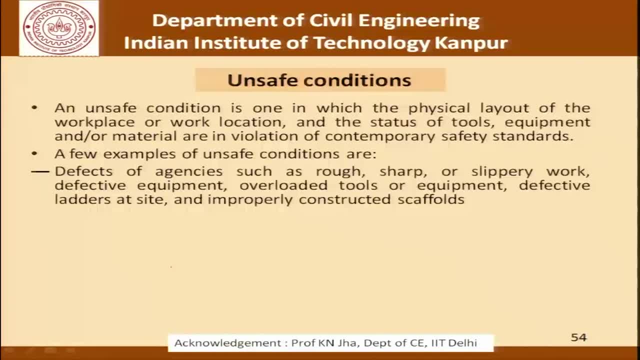 This what we have already seen, and few examples of these could be defects of agencies, such as rough, sharp or slippery work, defective equipment, overloaded tools or equipment, defective ladders at site, improperly constructed scaffolds, dress or apparel. hazards such as lack of protecting equipment and improper clothing. environmental hazards such as inadequate oil. 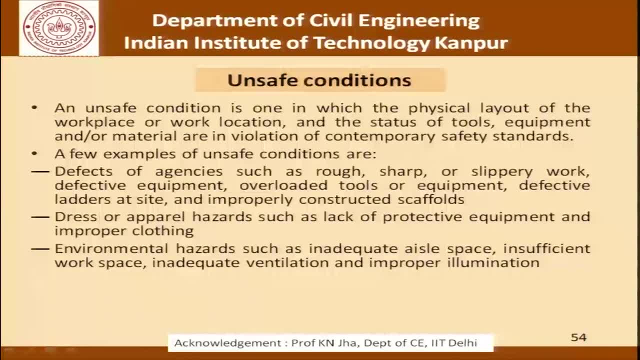 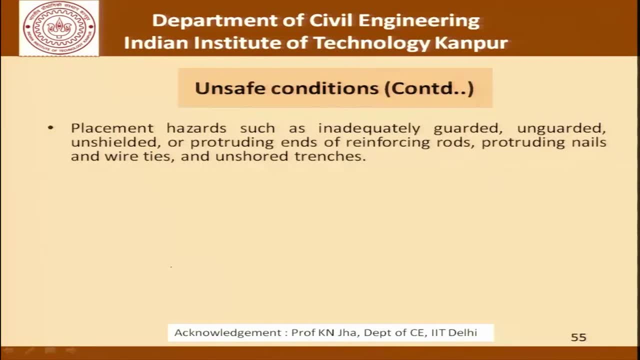 space, insufficient work space, inadequate ventilation and improper illumination. And if we continue with this list, it could be placement hazards such as inadequately guarded, unguarded, unshielded, protruding ends of enforcing bars, protruding nails, wire ties and unshoed trenches. 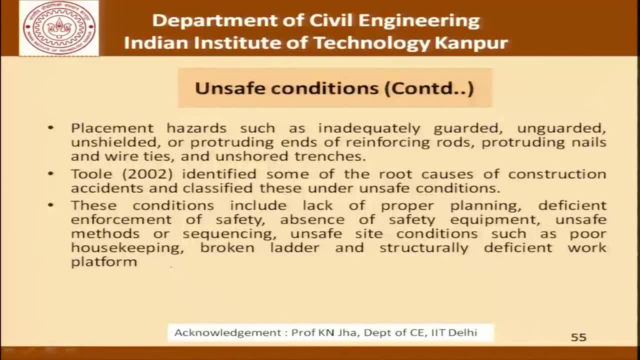 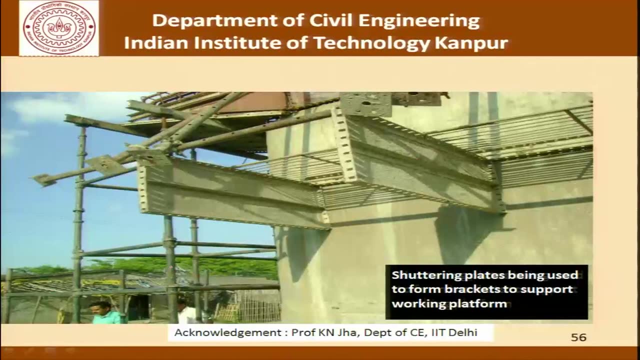 These conditions are basically due to lack of proper planning, deficient enforcement of safety, absence of safety equipment, unsafe methods or sequencing unsafe site conditions such as Under house keeping, broken ladders, structurally deficient work platforms and so on. Now let us take a look at some of the unsafe conditions and photographs from sites where 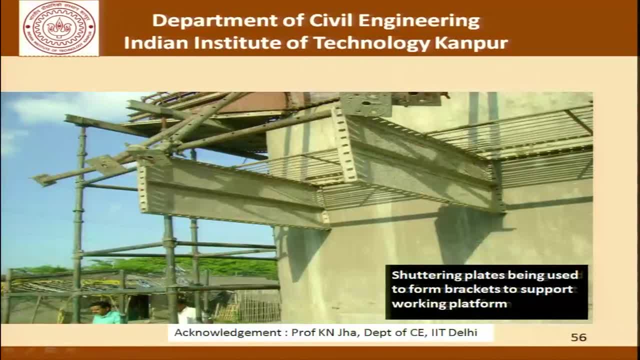 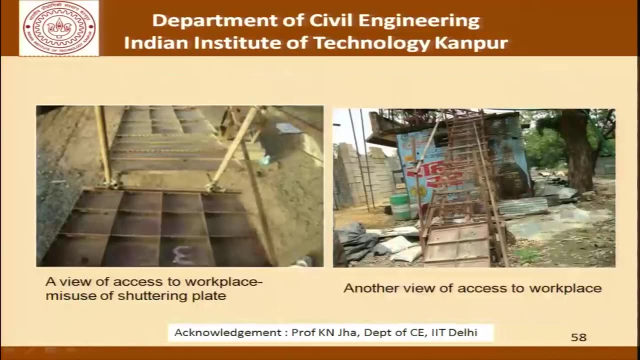 we will be able to clearly see how safety norms are violated. Here, for example, we see shuttering plates being used to form brackets to support platforms. Here we see shuttering plates being used as pedestals and, even worse, they are kept on loose soil. 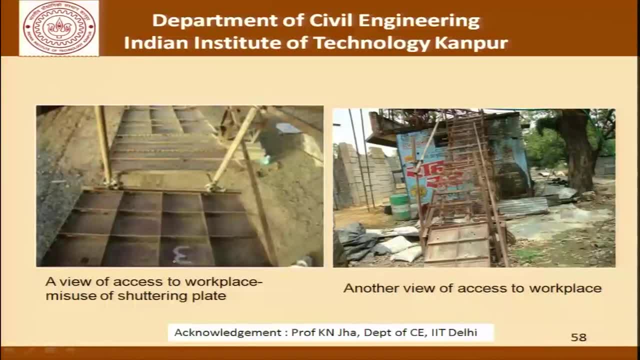 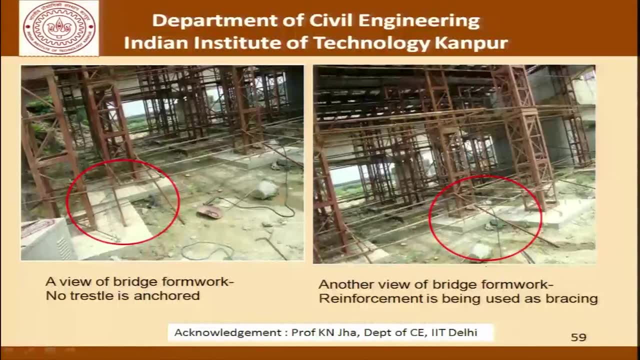 These pictures show a view of access to the workplace. Again, it is a misuse of shuttering plates. This is the view of a bridge formwork with trestles not anchored and another view where the bridge formwork reinforcement being used as bracings. 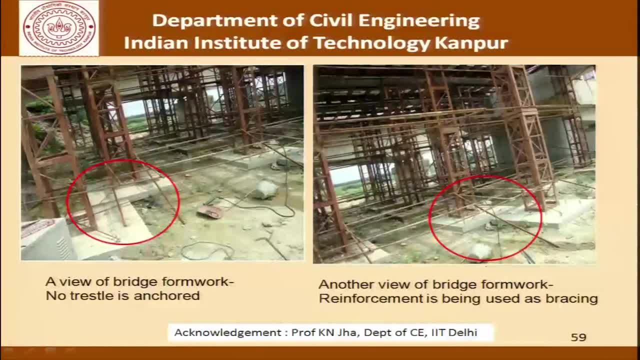 It is important to understand that, no matter what the worker does, the management must ensure a clean site. It is important for the execution team to have good house keeping and good practices being practiced at site and therefore such conditions are unsafe conditions arising out of misuse of shuttering plates. 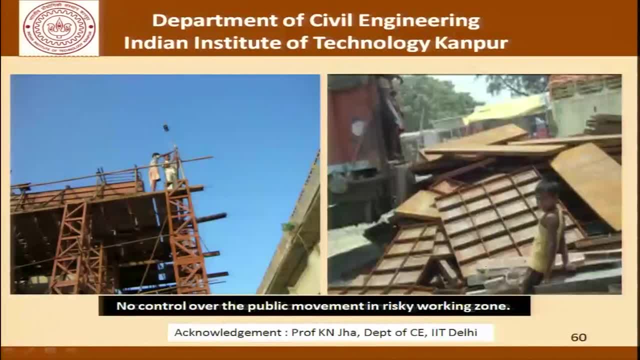 Now, in this case we see that there is absolutely no control on the public movement in a risky work zone. So obviously, if there is an accident in this case, it is not the worker who will be injured, but somebody who is not connected directly to the construction work at all. 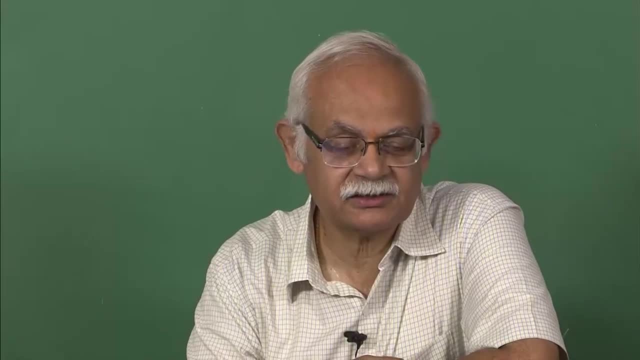 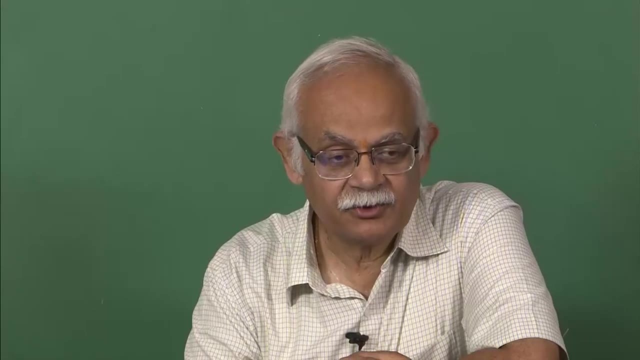 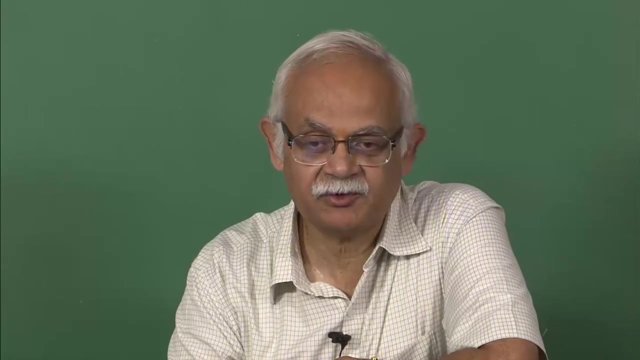 The question is whether it is the constructor's responsibility to also ensure that people who are not related, who are not trained, to enter the construction site. So this is the question: The construction site, should they be allowed free access? There have to be provisions, there have to be ways and means by which the site is barricaded. 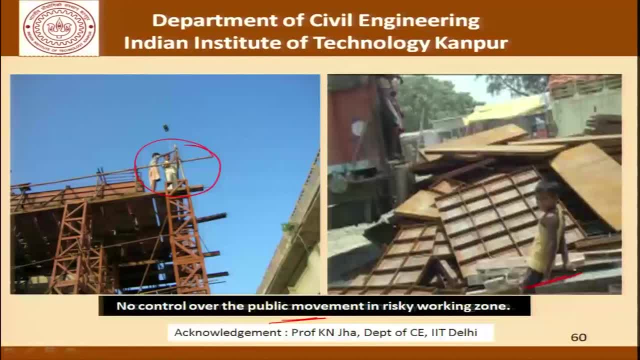 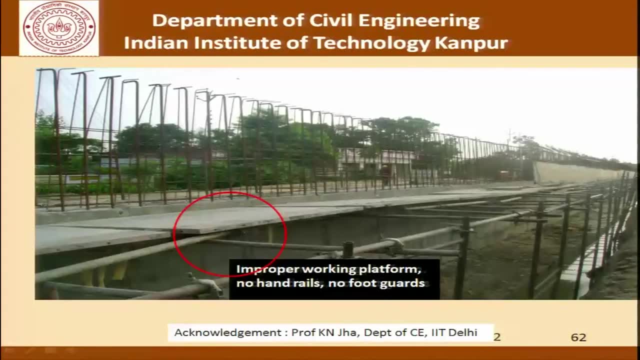 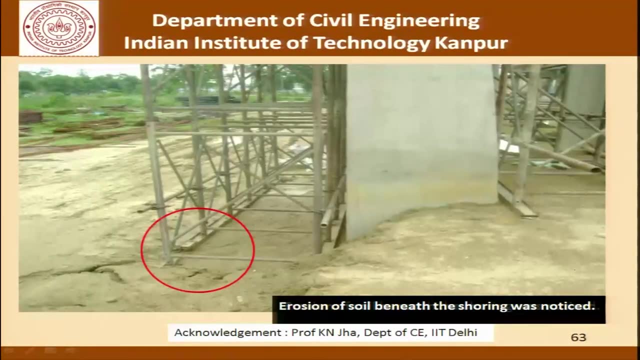 The same thing is here. we find a small boy standing among the shuttering plates. Here we find foot plates not in proper contact with concrete pedestals. We find working platforms with no handrails or foot guard. We find shoring where there is erosion of soil beneath. 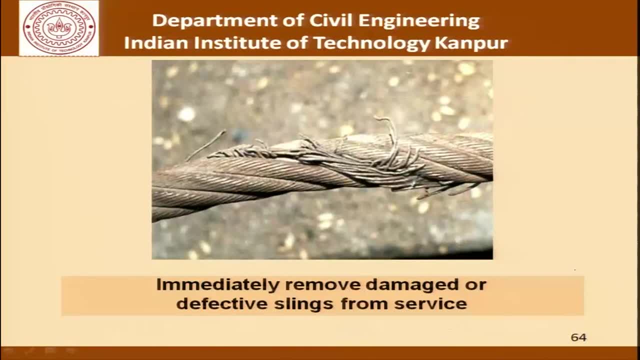 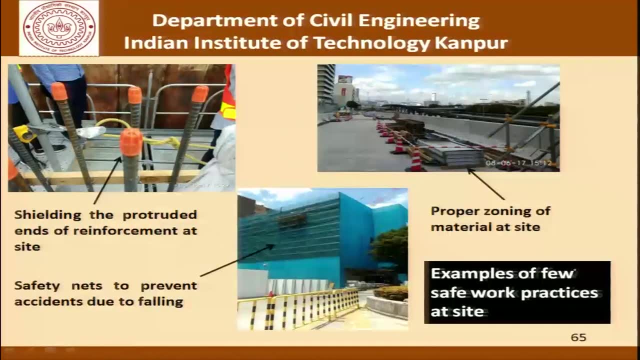 This is the case of a damaged sluice. This is the case of a damaged sluice. This is a work that needs to be loaded. This is proof of maintenance which needs to be removed from service Now. after seeing so many poor housekeeping slides, this is an example of a better management. 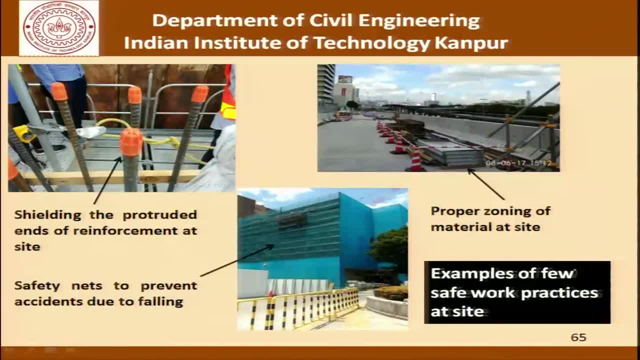 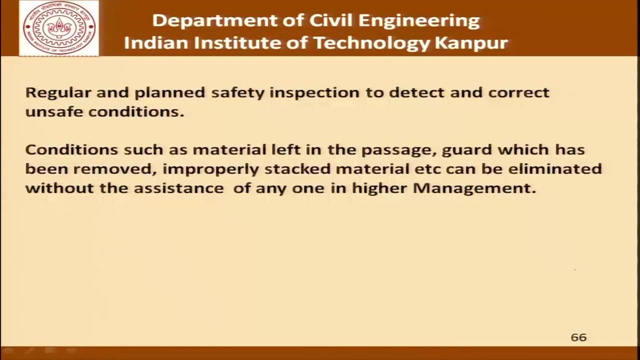 where there is shielding of protruding ends of reinforcement safety nets and proper zoning of the materials at sight. So it is not that it is not don't be done. It is only a matter of having the will to actually do it. Regular and planned safety inspection to detect and correct unsafe conditions are a very important. 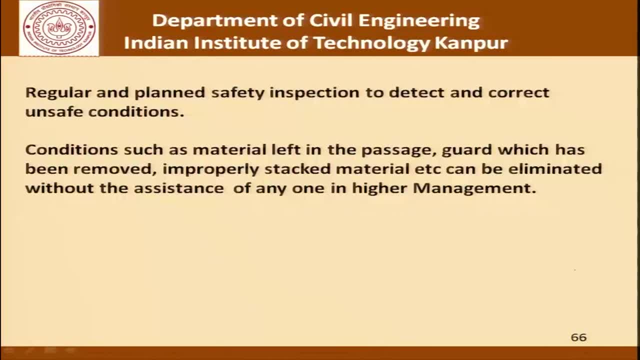 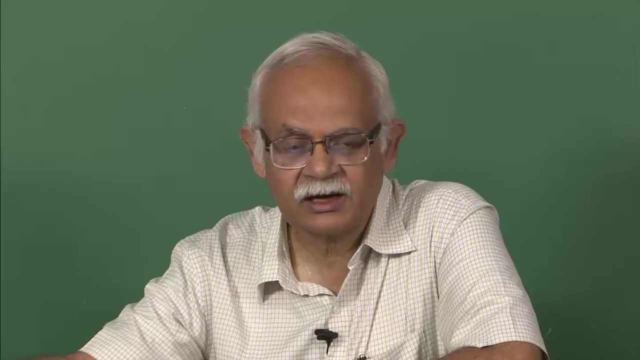 part responsibility that a culture is enforced at sites where unsafe conditions are not allowed to prevail. Conditions such as material left in the passage guard which has been removed. improperly stacked material can be eliminated without the assistance of anyone in higher management. It does not go right to the top of the company to introduce or to ensure compliance with. 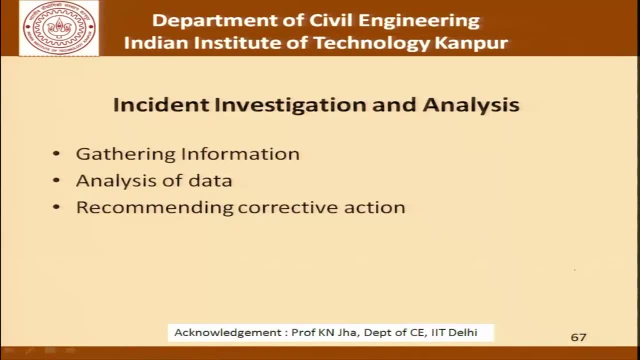 these simple things. One important part, before we close the discussion today, is that relating to incident investigation and analysis. There are three parts to this. one is gathering information, the other is analysis of data, and then it is recommending corrective action. This also comes into the ambit of the responsibilities of the safety group.